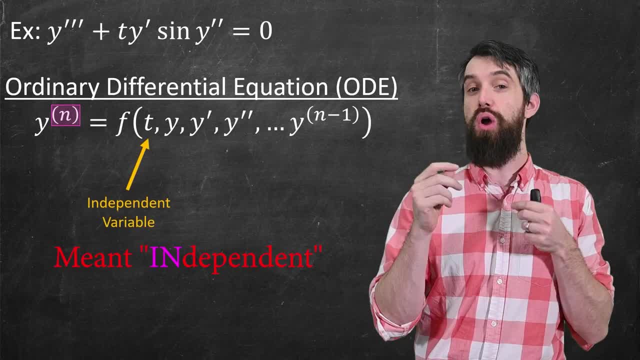 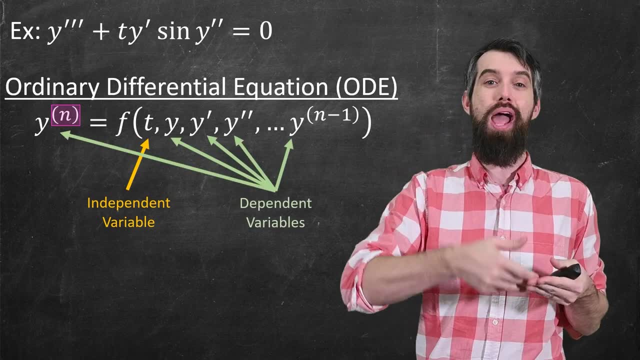 specified between a dependent variable that I'll call t- sometimes t, sometimes x- and a dependent variable, y, and its derivatives. So I'm going to start off with the nth derivative of y, y-prime, y-double-prime, all the way, potentially. 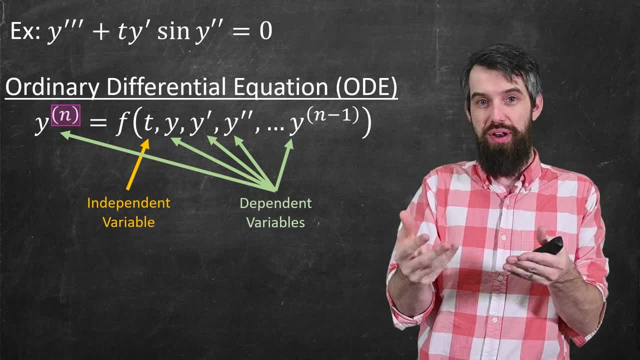 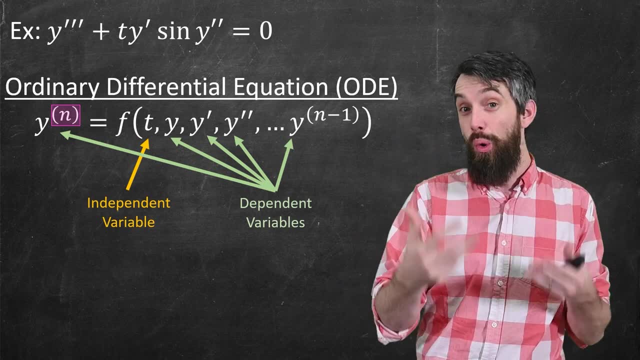 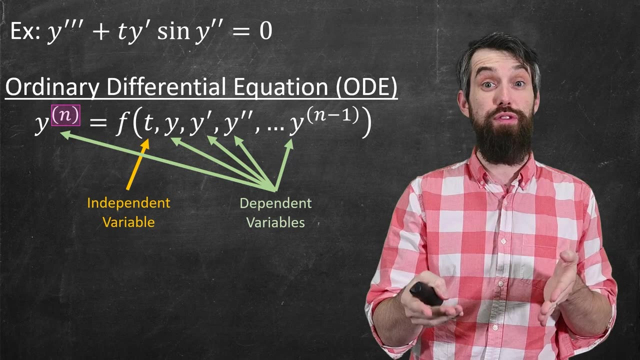 up to y, to the n-minus-1th derivatives, And so your nth derivative with respect to t depends on the previous derivatives, the lower order derivatives and the independent variable t. Now, differential equations have different types of properties, and one of them is referred. 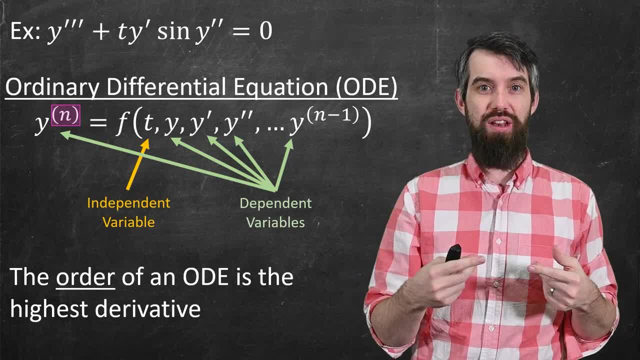 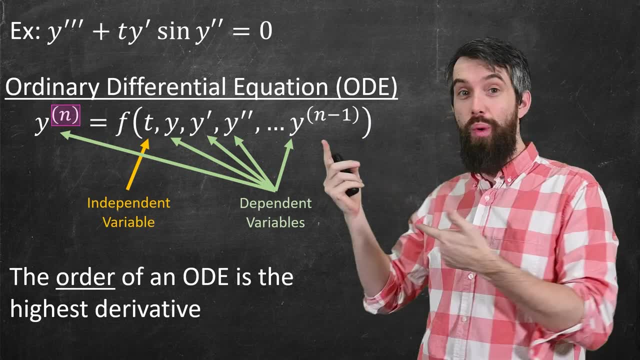 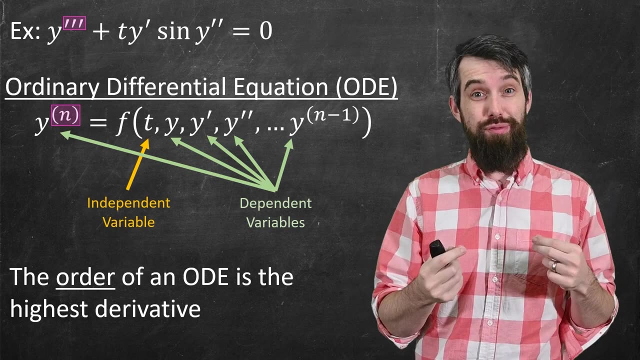 to as the order of a differential equation, And the order of a differential equation is just the highest derivative that appears. So in my example, where there was a y-triple-prime, that y-triple-prime is the highest order of a derivative, and so we say the order of that differential equation is 3.. 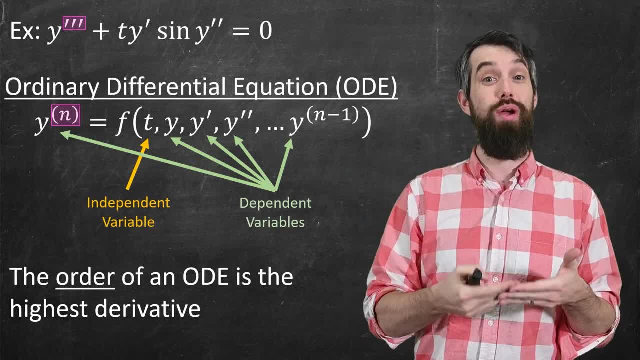 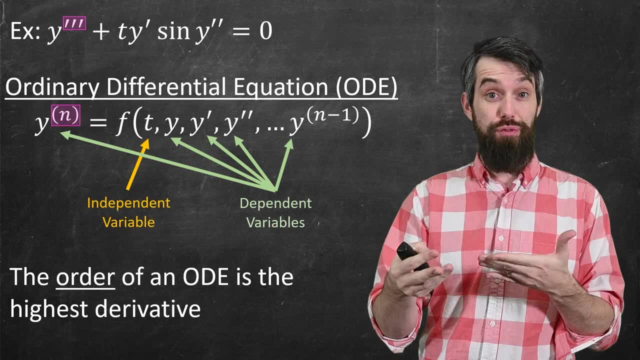 And in the general case that is an nth-order differential equation, The highest derivative that appears is the nth derivative And indeed order is going to be a distinguishing feature for us in our study of differential equations. We're going to begin by studying first-order differential equations, where there's only 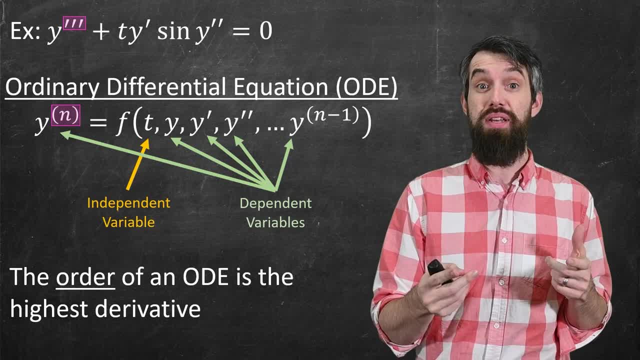 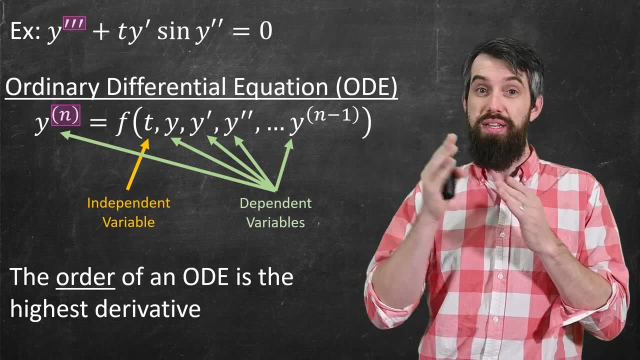 one derivative involved. This is going to take actually quite a bit of development, and then we'll move to higher-order differential equations after that. Now you'll notice that I called this an ordinary differential equation. So what are the other options? 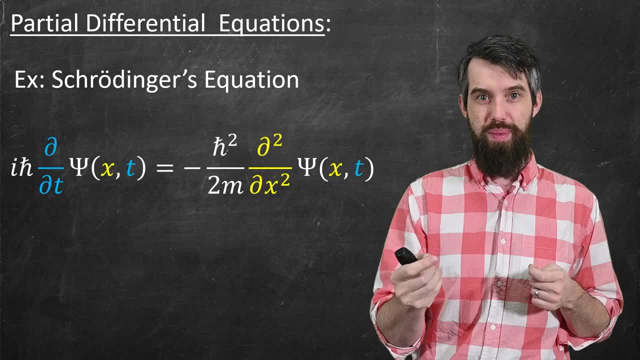 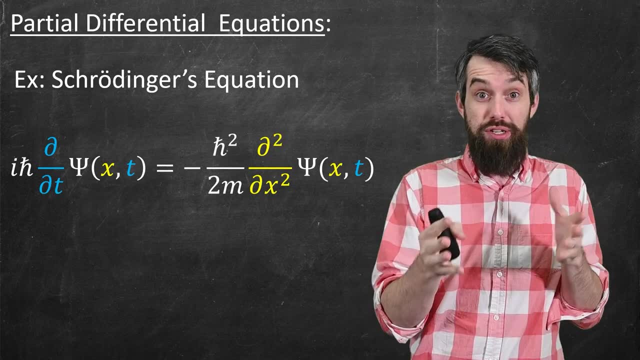 Now, we're not going to talk about these until quite a long time from now. but the other big category is so-called partial differential equations. In this equation- Schrodinger's equation from quantum mechanics, one of the most important differential equations that there is- we have some function that depends on both x and y-triples. 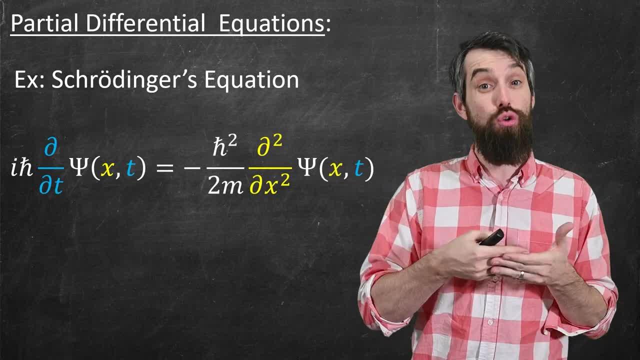 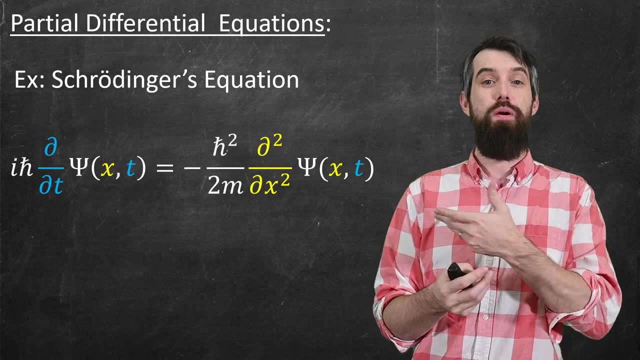 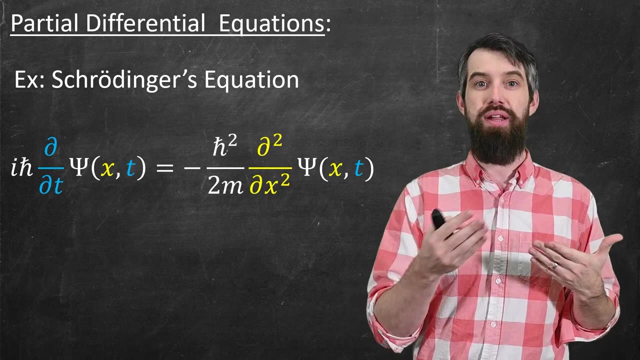 And then you have derivatives with respect to t and derivatives with respect to x. They're partial derivatives. now, So when your differential equation is involving multiple variables and they're partial derivatives, then we call it a partial differential equation. If there's just one independent variable, then it's an ordinary differential equation. 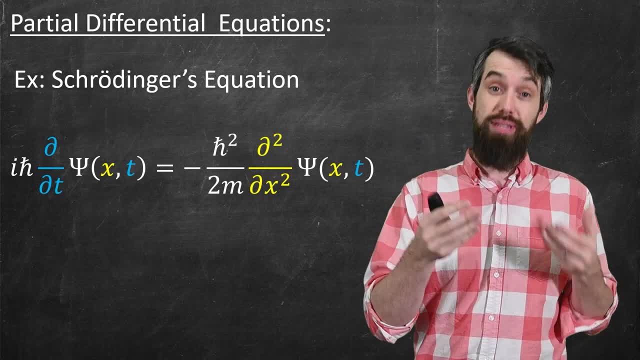 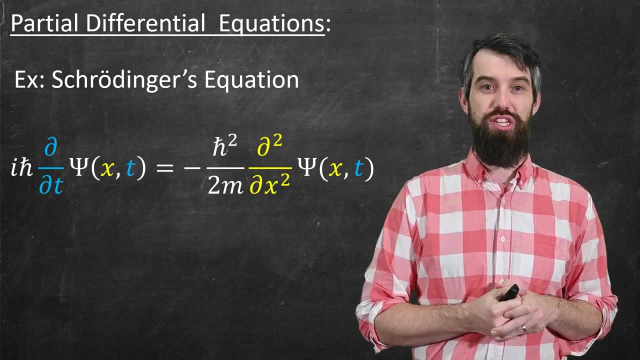 And indeed we're going to be focusing on ordinary differential equations, at least for now. The other complexity that can happen- and again this is going to be something for the future- is systems of differential equations Where you have not one but multiple different differential equations. 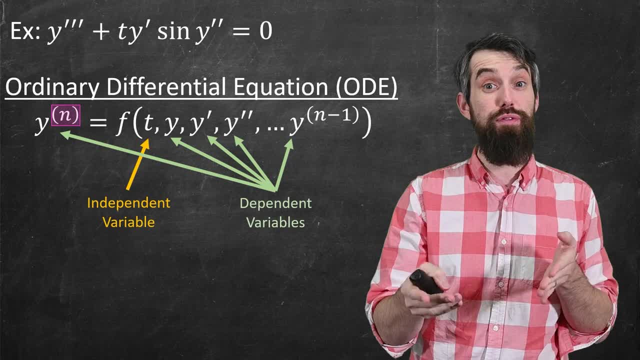 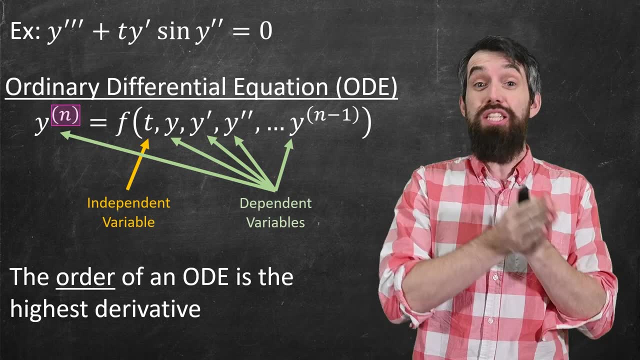 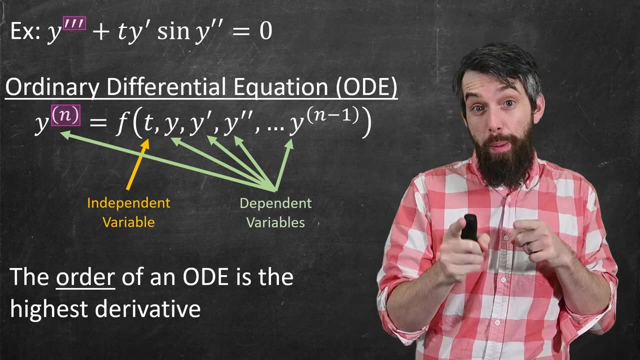 Now, differential equations have different types of properties, and one of them is referred to as the order of a differential equation. And the order of a differential equation. The order of a differential equation is just the highest derivative that appears. So in my example, where there was a y triple prime, that y triple prime is the highest. 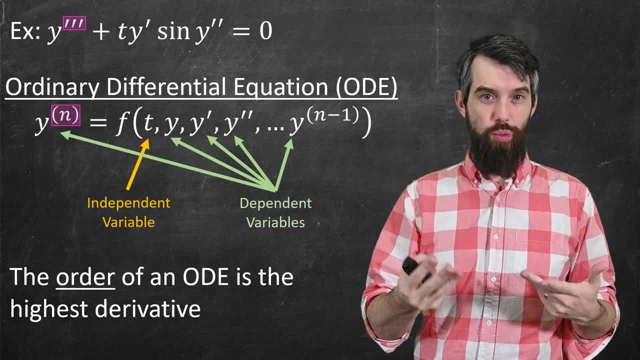 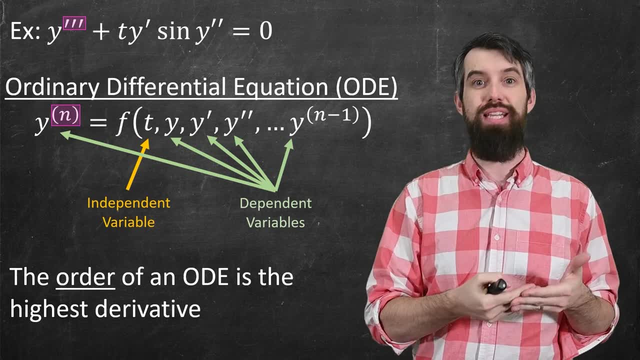 order of a derivative. and so we say the order of that differential equation is 3.. And in the general case that is an nth order differential equation. The highest derivative that appears is the nth derivative. And indeed order is going to be a distinguishing feature for us in our study of differential 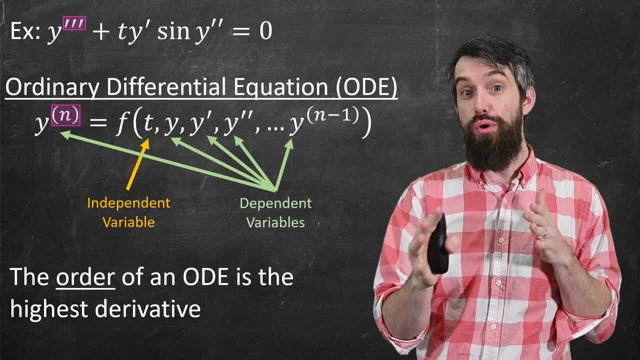 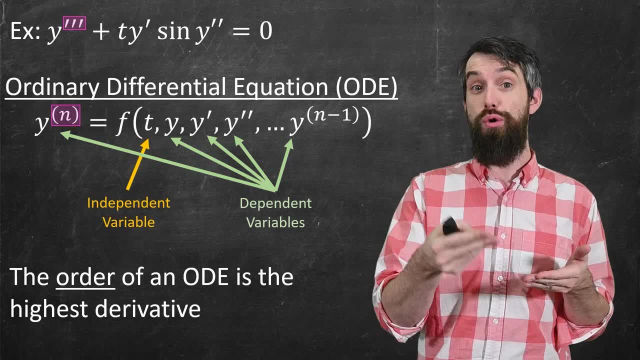 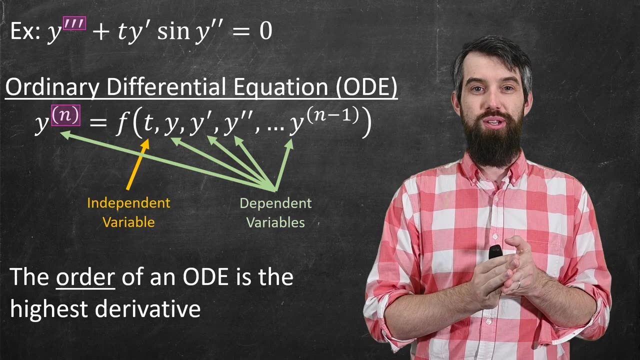 equations. We're going to begin by studying First order differential equations where there's only one derivative involved. This is going to take actually quite a bit of development, and then we'll move to higher order differential equations after that. Now you'll notice that I called this an ordinary differential equation. 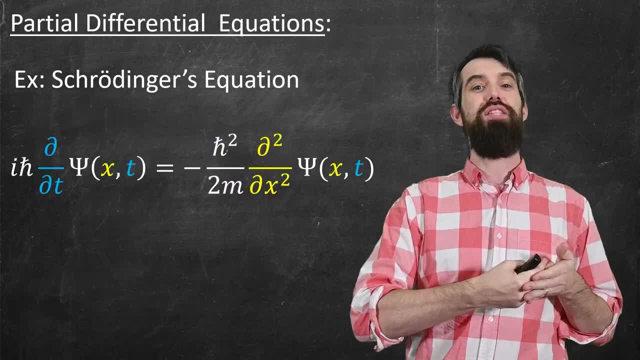 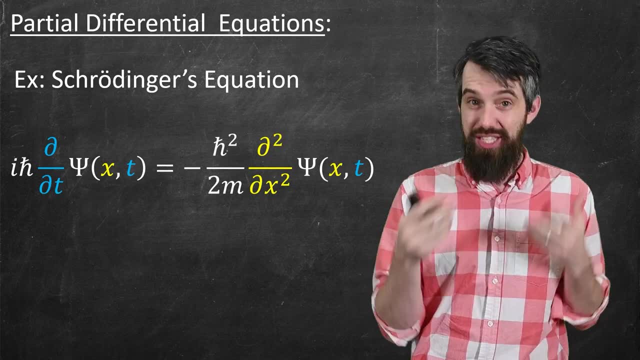 So what are the other options? Now, we're not going to talk about these until quite a long time from now, but the other big category is so-called partial differential equations. In this equation, Schrodinger's equation from quantum mechanics, one of the most important- 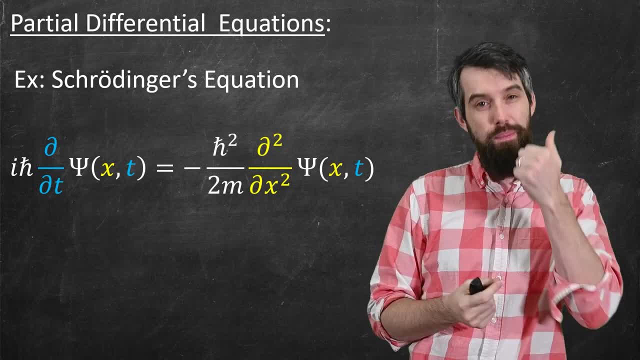 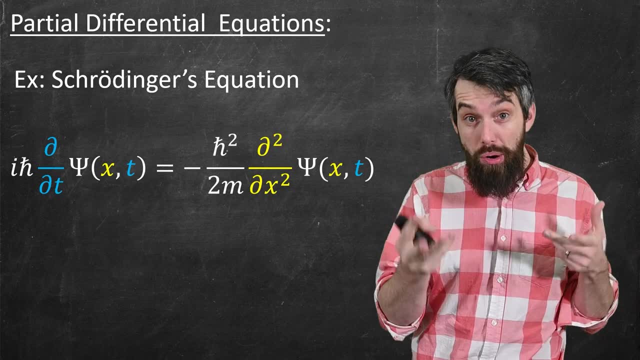 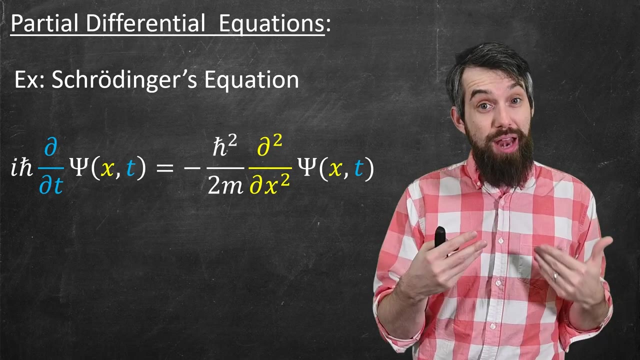 differential equations that I've ever studied. We have some function that depends on both x and t, and then you have derivatives with respect to t and derivatives with respect to x. They're partial derivatives. now, So, when your differential equation is involving multiple variables and they're partial derivatives, 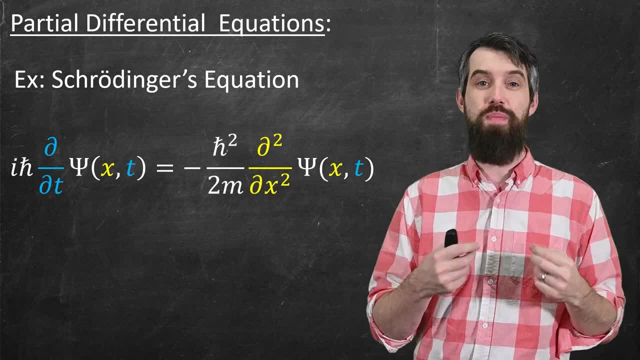 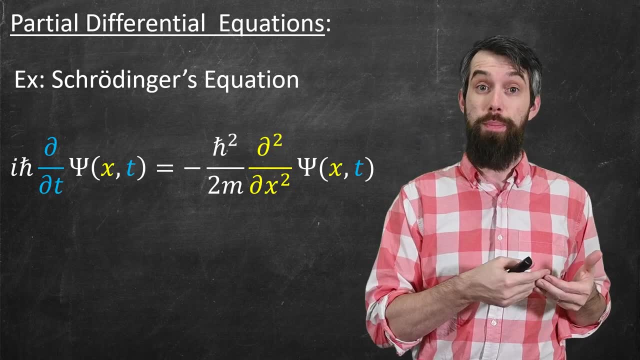 then we call it a partial differential equation. If there's just one independent variable, then it's an ordinary differential equation And indeed we're going to be focusing on ordinary differential equations, at least for now. The other complexity that can happen in a partial differential equation is that it's 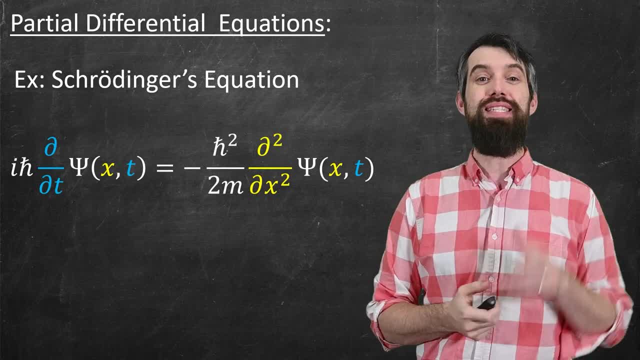 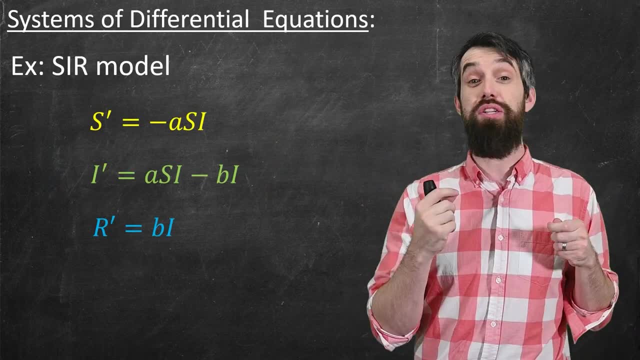 a partial differential equation- And again, this is going to be something for the future- is systems of differential equations where you have not one but multiple different differential equations. These are the equations for the SIR model that helps us study pandemics. 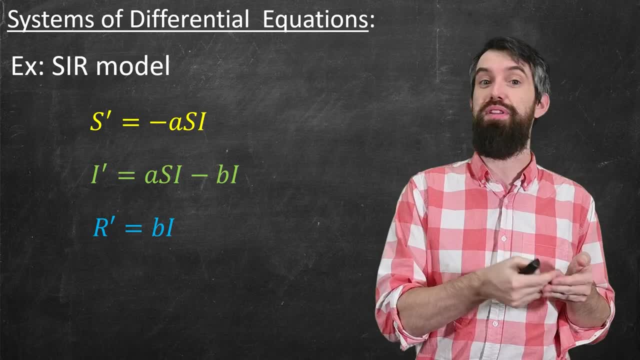 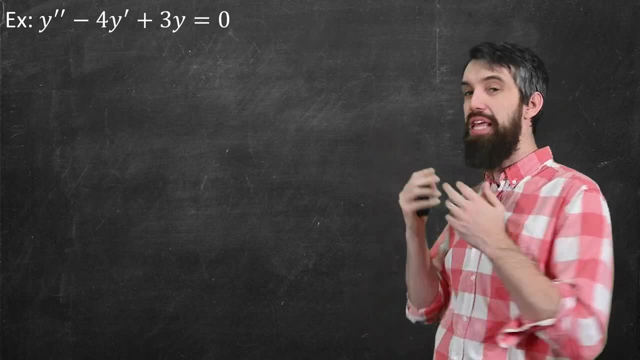 I actually have a couple of videos on this model, this system of differential equations, so you're welcome to check that out if you so wish. Regardless, our focus is going to be on ordinary differential equations like this one. Okay, so now that you have a differential equation, what can you do with it? 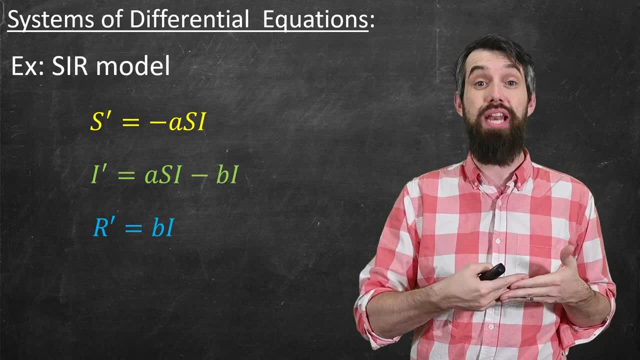 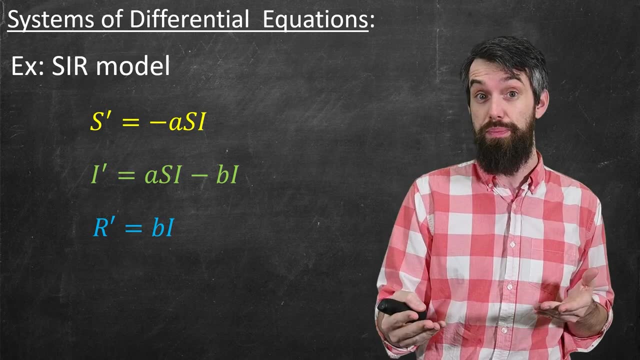 These are the equations for the S-I-R model that helps us study pandemics. I actually have a couple of videos on this model, this system of differential equations, so you're welcome to check that out if you so wish. Regardless, our focus is going to be on ordinary differential equations like this one. 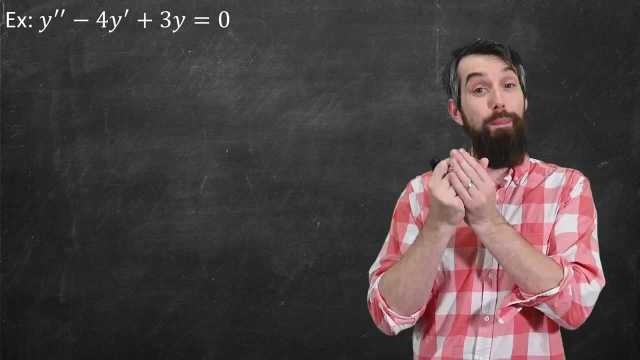 Okay. so now that you have a differential equation, what can you do with it? Well, the main thing we're trying to do is to solve a differential equation. So what exactly does that mean? Take, for example, a differential equation. 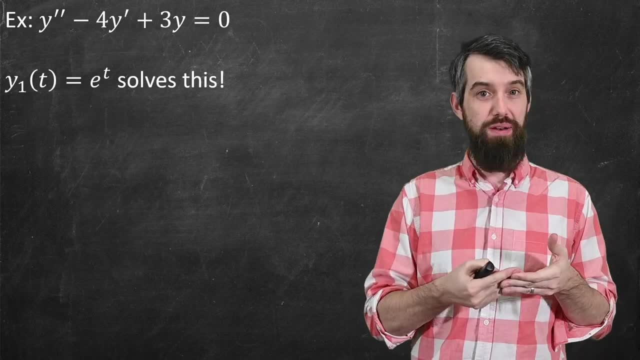 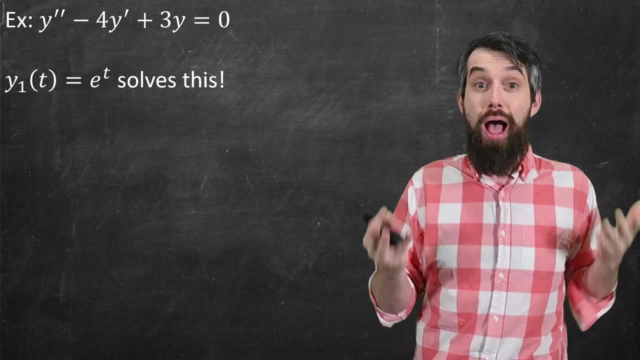 For instance, the function e to the t. I'll call this y1, because this is going to be the first of multiple solutions to this differential equation. My claim is that e to the t solves this equation. How do I know? Well, I'm going to plug it in. 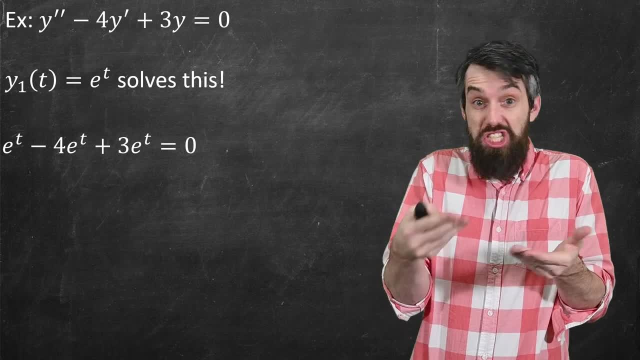 And I'm going to see that if I plug that in, so 2 to the riz of e to the t is just e to the t, Then I subtract off one derivative of e to the t times 4, which is just 4 e to the t. 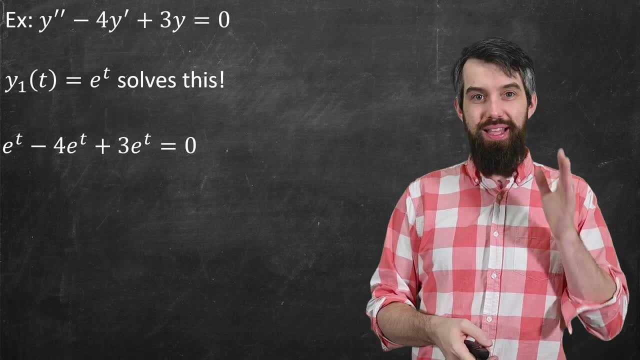 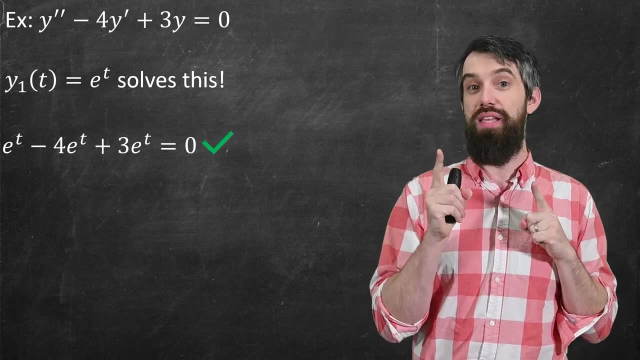 And then plus 3 times, plug it in: e to the t, and indeed e to the t, minus 4 e to the t plus 3 e to the t. Yeah, that adds up to 0.. So, yes, this satisfies the differential equation. 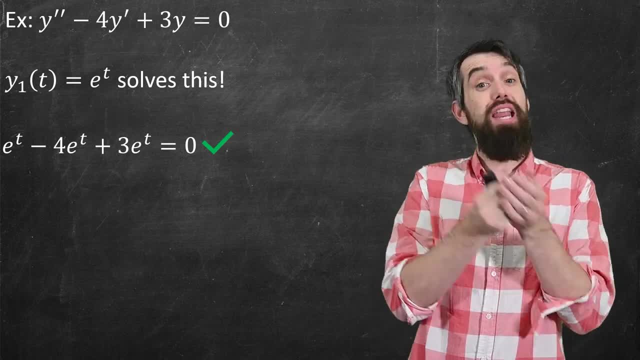 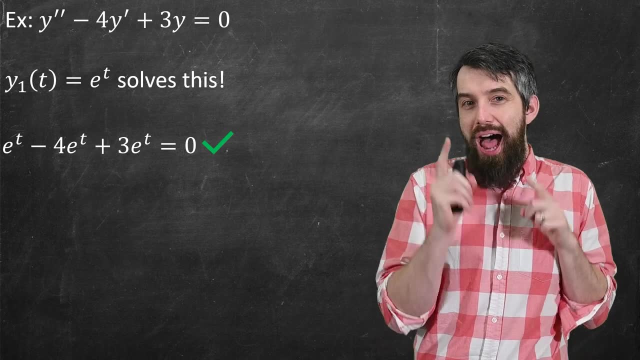 That is, I take this function, I plug it into the differential equation And if it satisfies it, then we're going to call it a solution. But I want you to note that in addition I could put some other constant c out, the 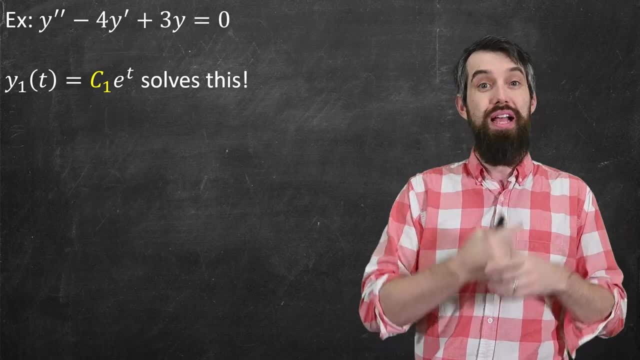 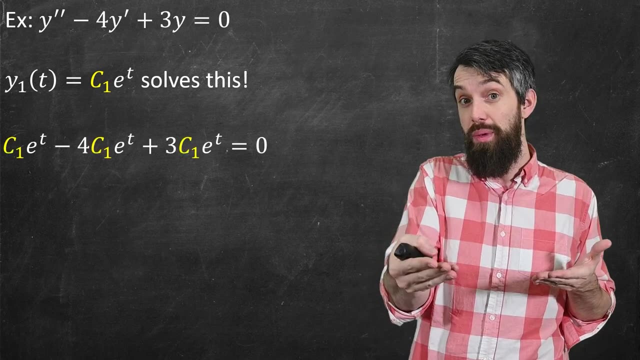 front of it some c1, because this is the first function I can talk about. c1 e to the t And the equation is exactly the same. I mean, constants just come out of derivatives, So it's just a c1 in front of every term. 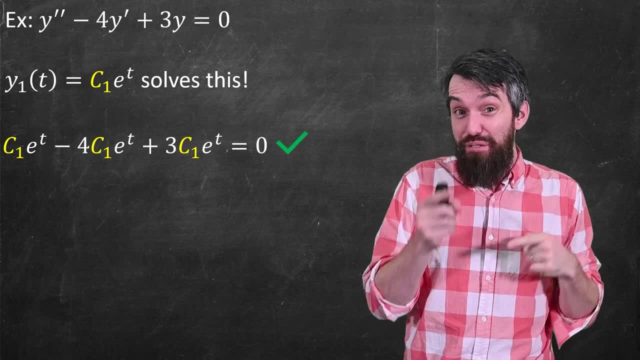 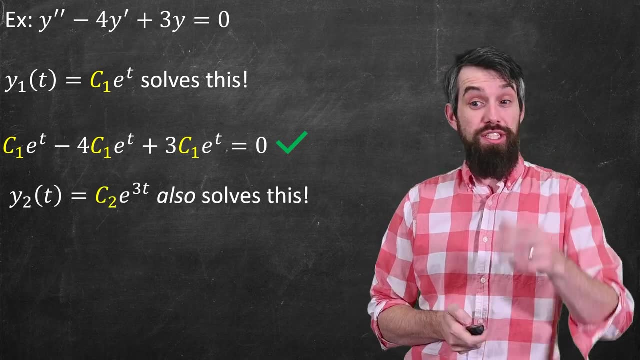 And so that adds up to 0 in just the same way. So we already have an infinite family of solutions. but it's actually even more complicated than that. Consider what I'll now call y2, which is some constant times e to the 3t. 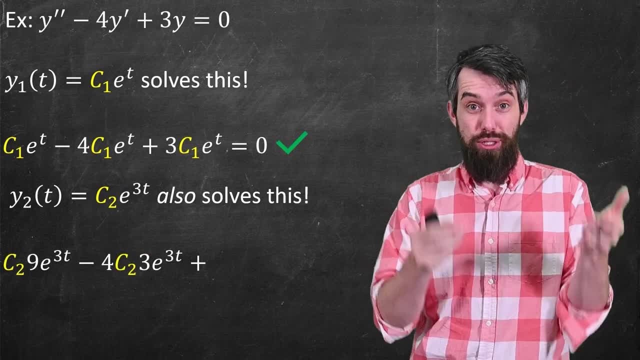 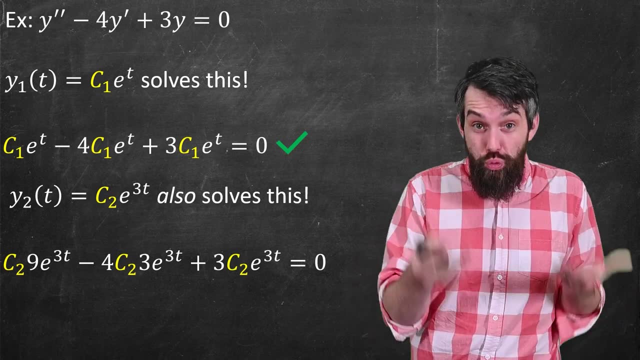 No longer e to the t, e to the 3t. Well, it's also a solution, Indeed. plug it in the same way and you're going to get 9 times the constant e to the 3t, then minus 12, the constant e to the 3t, and then plus 3, the constant times e to the. 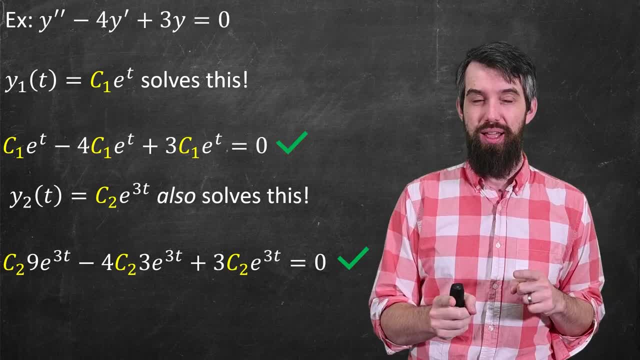 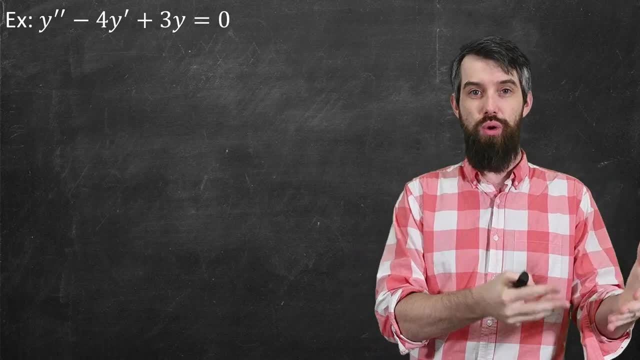 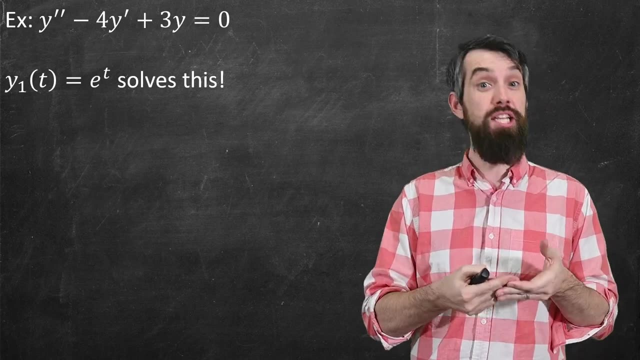 Well, the main thing we're trying to do is to solve the differential equation. So what exactly does that mean? Take, for instance, the function e to the t. I'll call this y1, because this is going to be the first of multiple solutions to this. 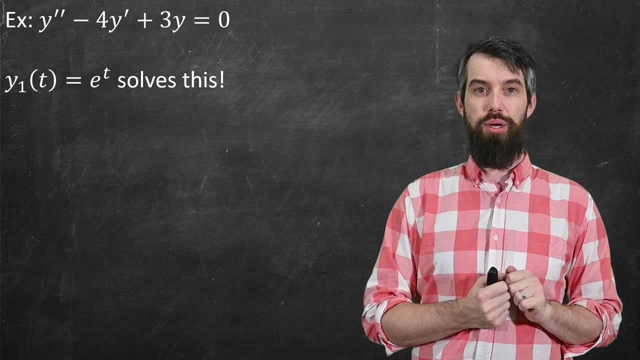 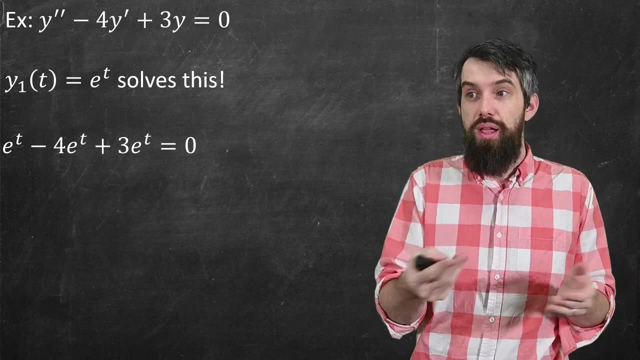 differential equation. My claim is that e to the t solves this equation. How do I know? Well, I'm going to plug it in and I'm going to see that, if I plug that in, so 2 to the t is just e to the t. 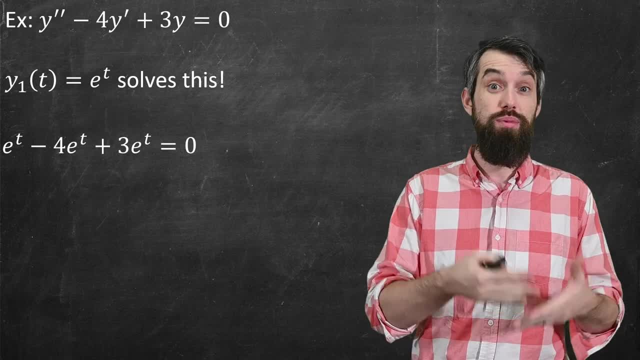 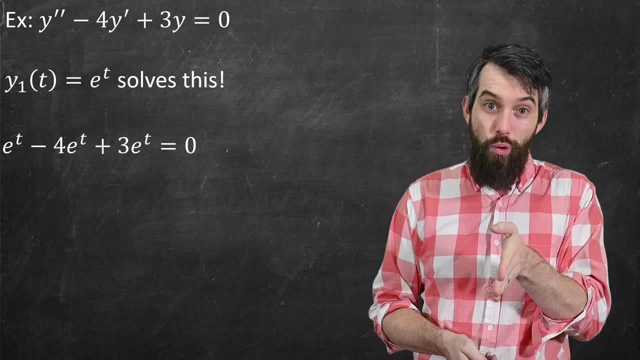 Then I subtract off one derivative of e to the t times 4, which is just 4e to the t, And then, plus 3 times, plug it in e to the t, and indeed e to the t minus 4, e to the t plus 3, e to the t. yeah, that adds up to zero. so 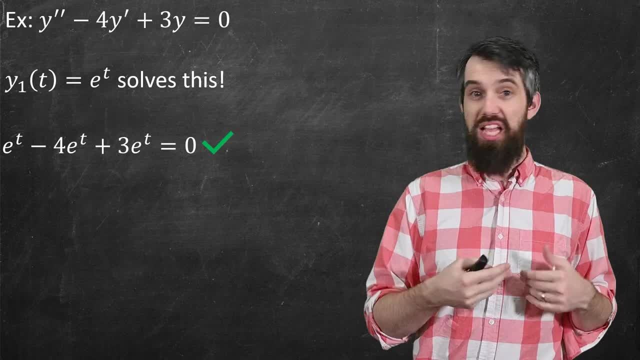 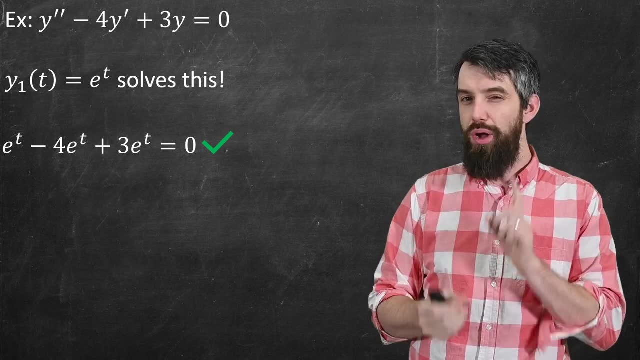 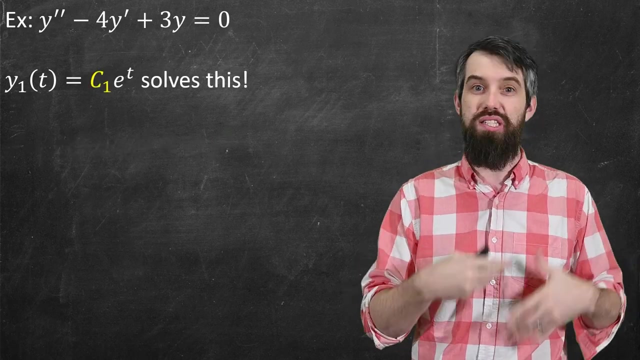 yes, this satisfies the differential equation. that is, i take this function, i plug it into the differential equation and if it satisfies it, then we're going to call it a solution. but i want you to note that in addition, i could put some other constant c out the front of it, some c1, because 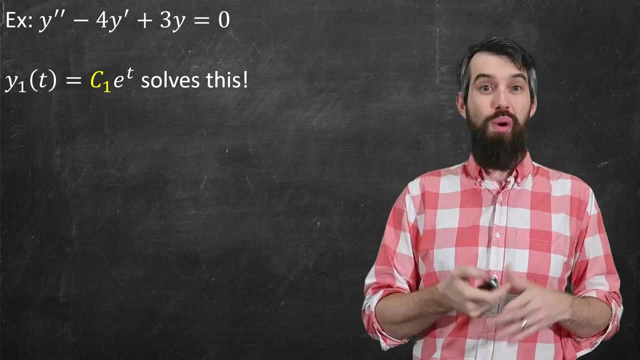 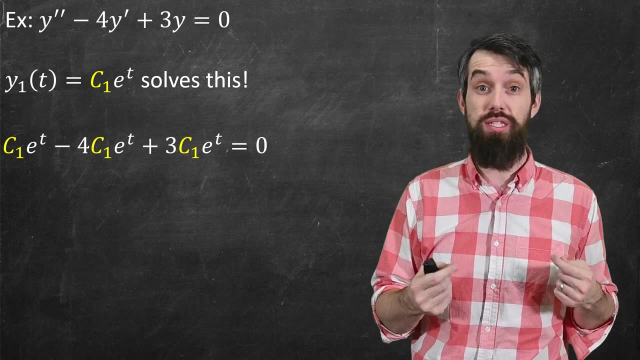 this is the first function i can talk about: c1, e to the t, and the equation is exactly the same. i mean constants just come out of derivatives, so it's just a c1 in front of every term and so that adds up to zero in just the same way. so we already have an infinite family of solutions, but it's. 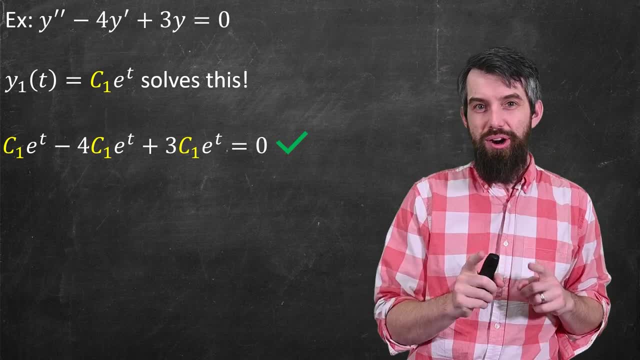 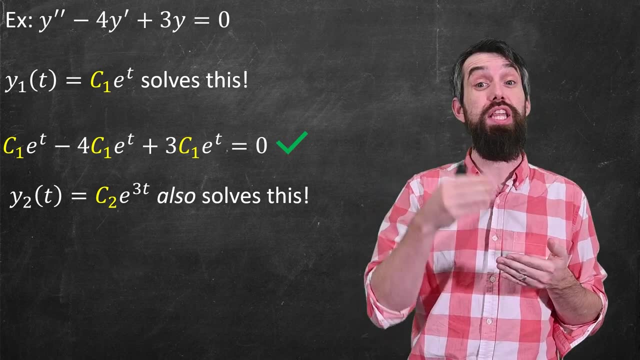 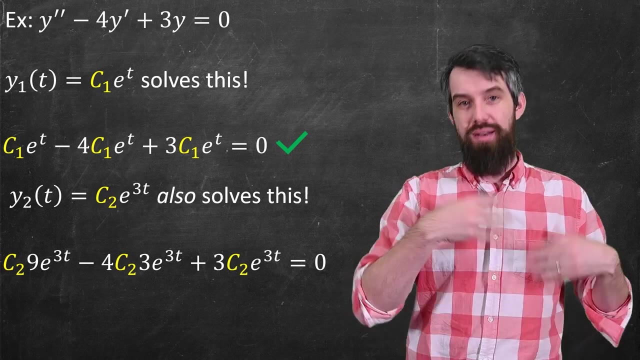 actually even more complicated than that. consider what i'll now call y2, which is some constant times e to the 3t. no longer e to the t, e to the 3t. well, it's also a solution, indeed. plug it in the same way and you're going to get 9 times the constant e to the 3t, that minus 12. 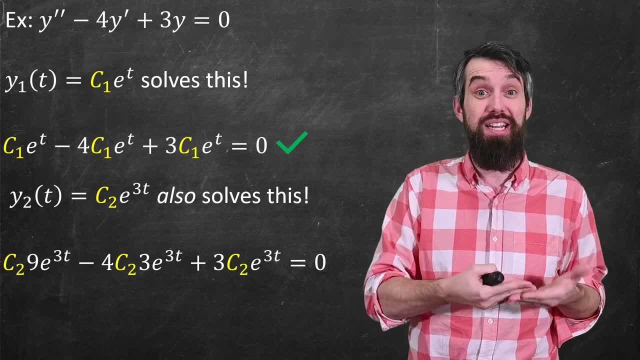 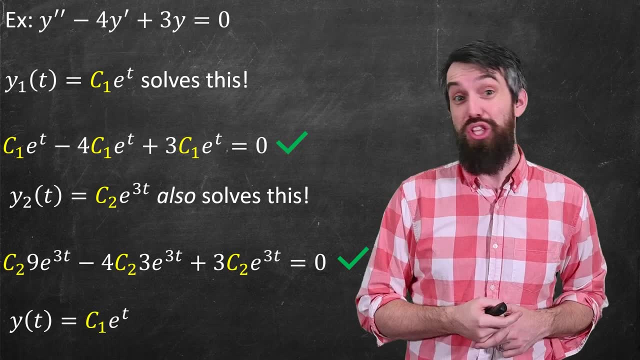 the constant e to the 3t and then plus 3 the constant times e to the 3t, which adds up to zero. it's again a solution. so we've got a y1 and a y2, and then i should leave it to you to verify if you. 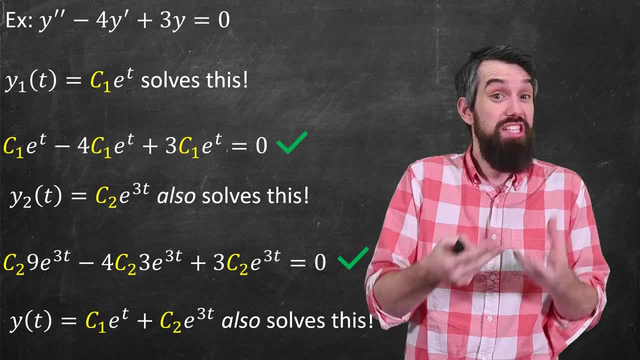 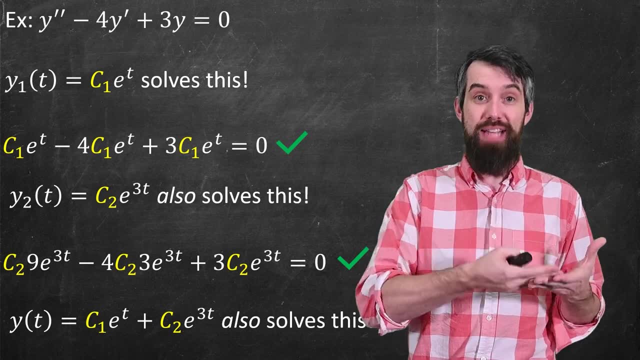 wish that any combination, like if you add those two, that it's also going to be a solution. this is because derivatives are linear- operators is one way to put it. so the sum of them is going to result in the sum of the solution. zero plus zero is just going to be zero. and now i've gotten. 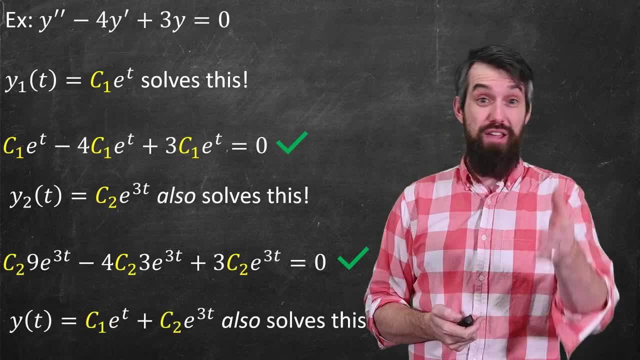 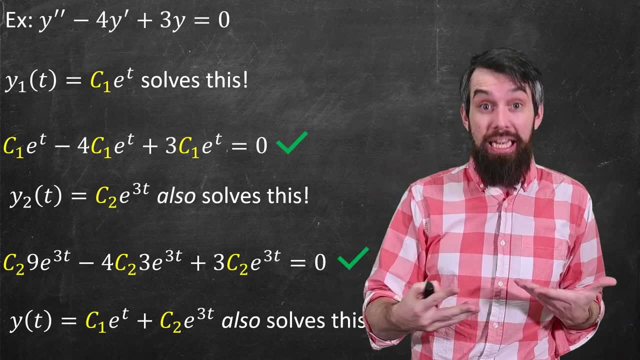 So we've got a y1 and a y2.. And then I'll actually leave it to you to verify, if you wish, that any combination, like if you add those two, that it's also going to be a solution. This is because derivatives are linear. operators is one way to put it. 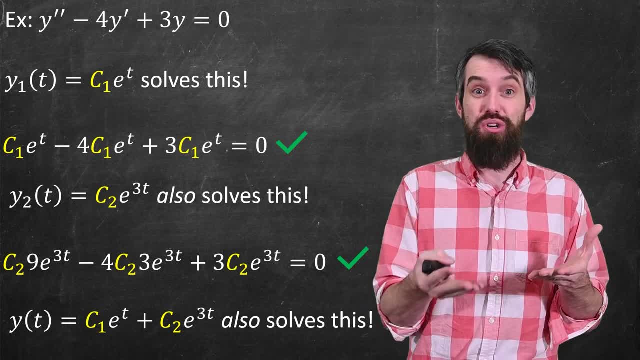 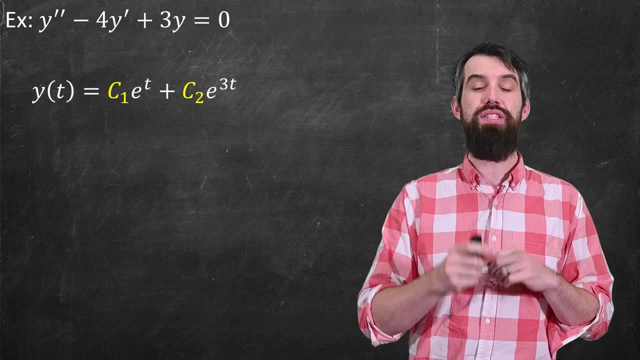 So the sum of them is going to result in the sum of the solution. 0 plus 0 is just going to be 0. And now I've gotten something that I'm going to isolate and refer to as the general solution. The general solution contains every point. 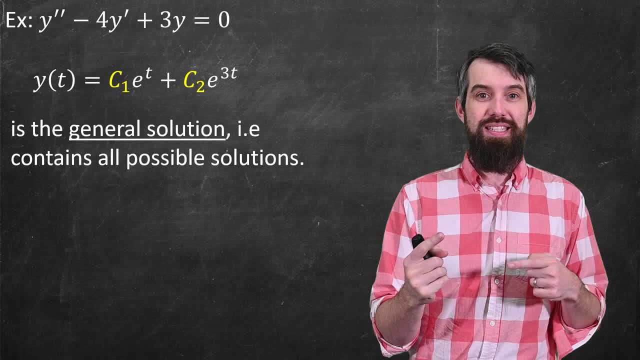 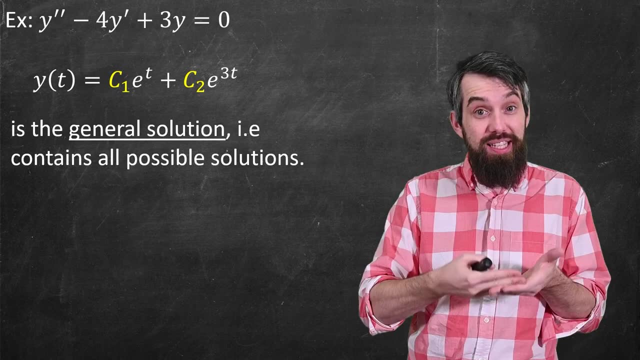 It's just a possible solution to this differential equation. That is, any possible solution to this differential equation can be written as the combination of c1 times the e to the t and c2 times e to the 3t for different values of those constants. 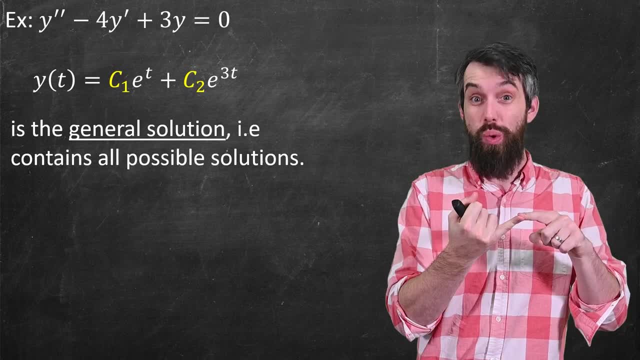 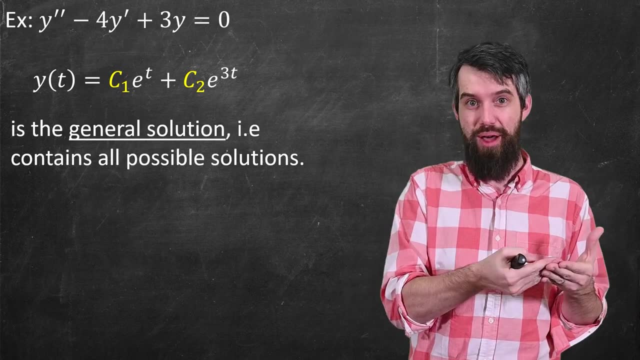 But OK, there's a lot of questions here, like: how did I know what those solutions were And how do I know that all of the solutions can be written in this way? Perhaps there's many other solutions that I haven't written down. 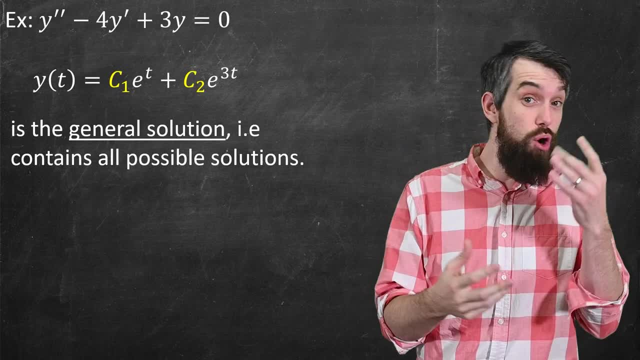 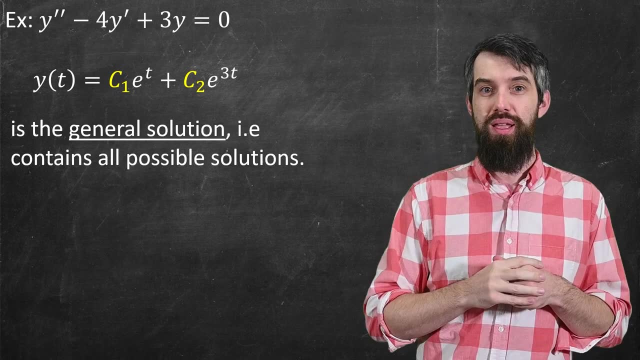 Now to the question of how do you find these solutions? How did I know e to the t and e to the 3t? This is a subject of our course. We are going to study that later on in later videos in this course. 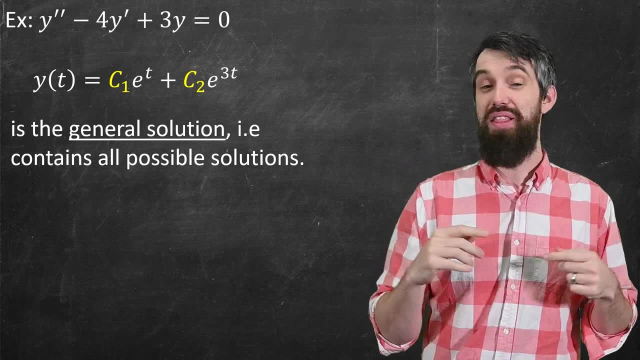 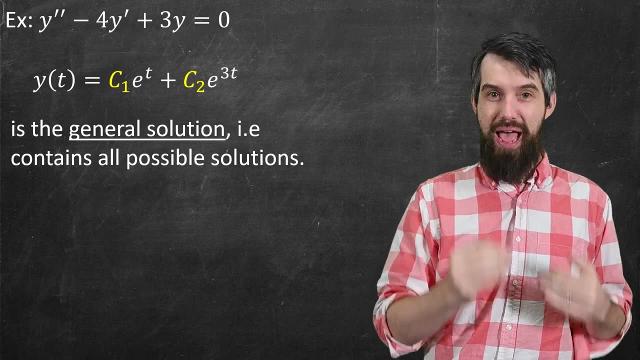 But for now, we can actually use technology to help us out, And the actual technology we're going to use comes from- and I'm very proud to say it- the first official sponsor of this math channel, which is Maple. What I can do with Maple Calculator, which is an app that you can install on your phone. 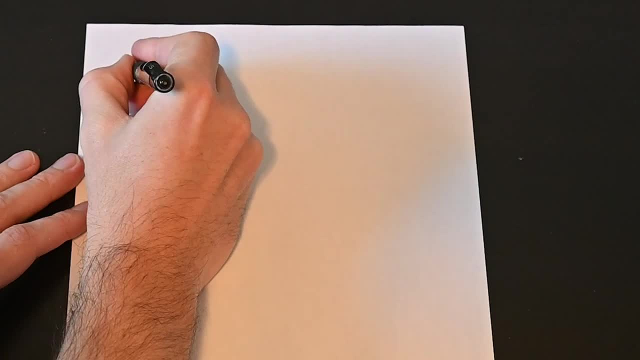 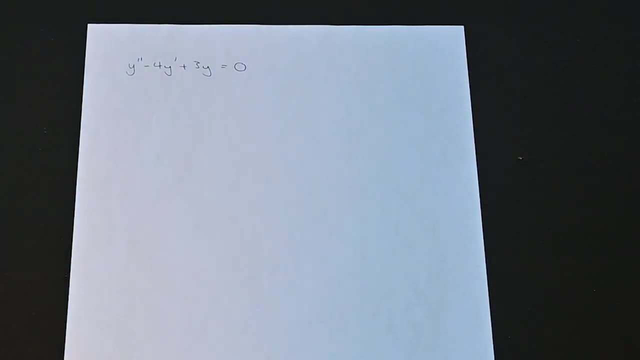 and the links are down in the description- is: I can just handwrite out the differential equation that I've written down. That's what I'm trying to study. So I can handwrite out: y, double prime minus 4y, prime plus 3y equal to zero. 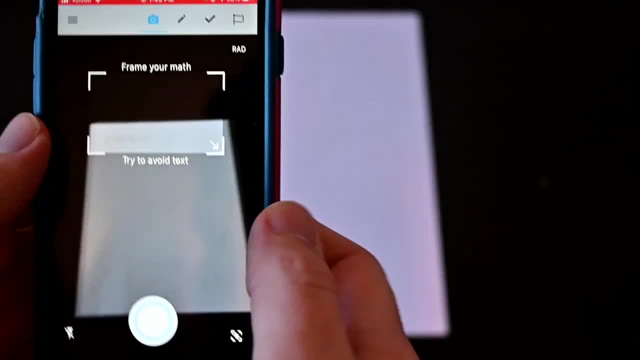 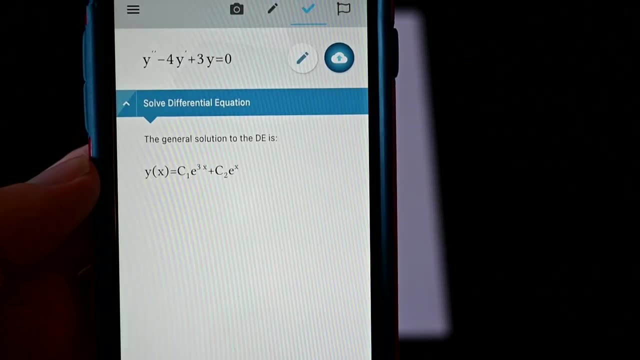 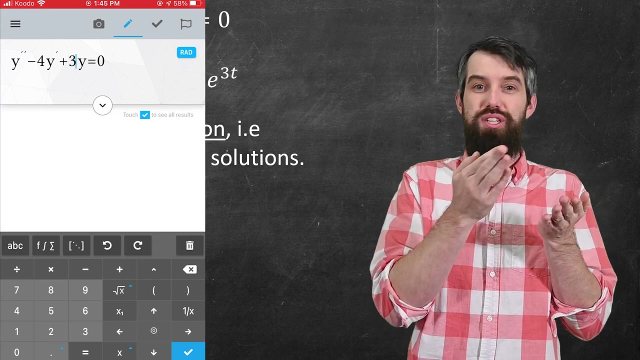 Then if I open the app, I can hit the camera button and I can just take a picture of my equation and the Maple Calculator will interpret it And look what it does: It automatically spits out the general solution to this differential equation. If you didn't want to bother with taking a photo, it's also totally fine for you to type. 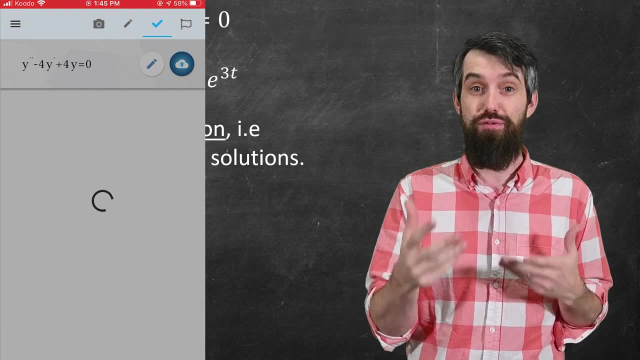 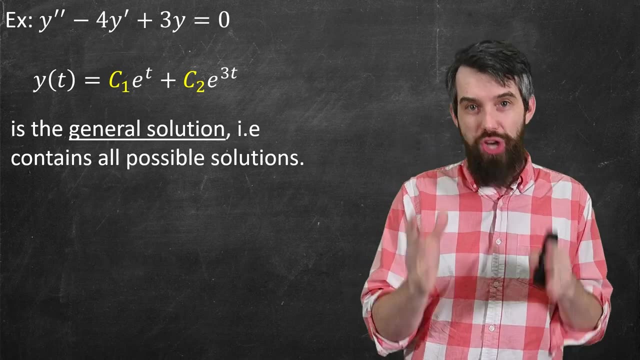 it in and to change the constants and see what the solutions are to any differential equation that you're interested in. And it's nice to know that, according to the Maple Calculator, this is all of the solutions. This is the general solution. Indeed, there's going to be a lot of theory that we'll develop later in the course, as 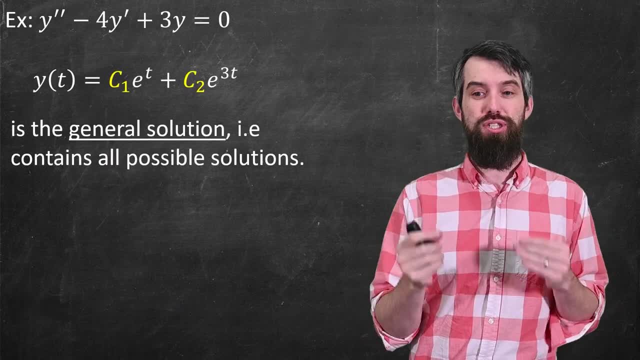 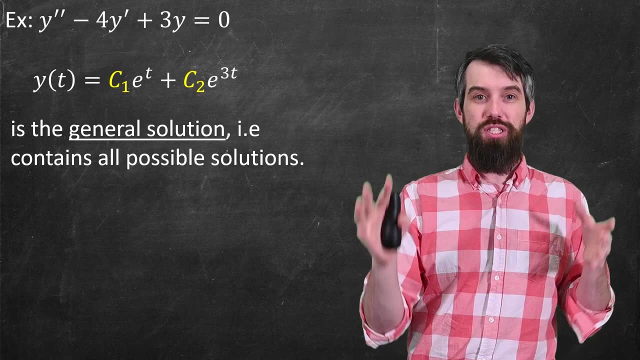 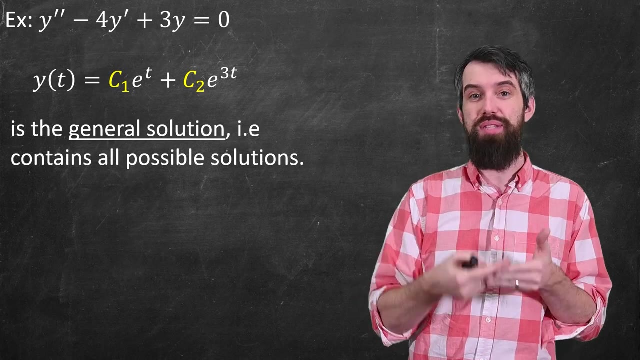 over to the general solution. the general solution contains every possible solution to this differential equation. that is, any possible solution to this differential equation can be written as the combination of c1 times the e to the t and c2 times e to the 3t for different. 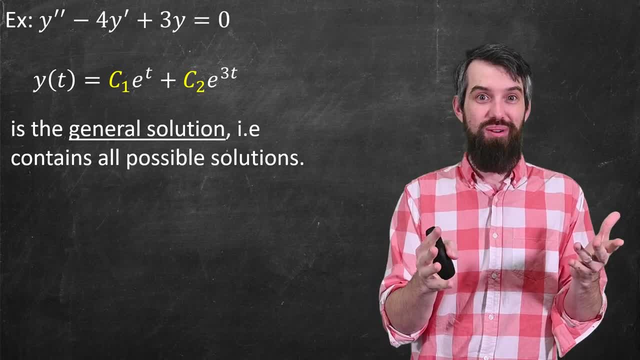 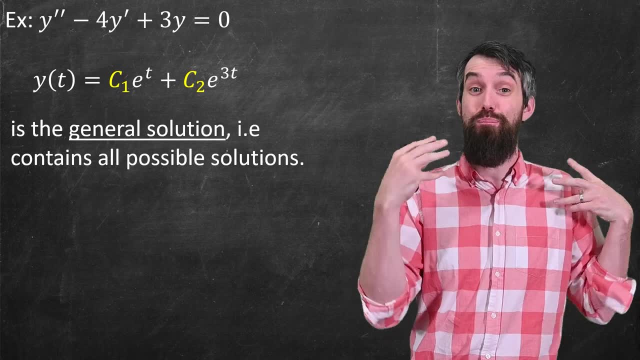 values of those constants. but okay, there's a lot of questions here, like: how did i know what those solutions were and how do i know that all of the solutions can be written in this way? perhaps there's many other solutions that I haven't written down. 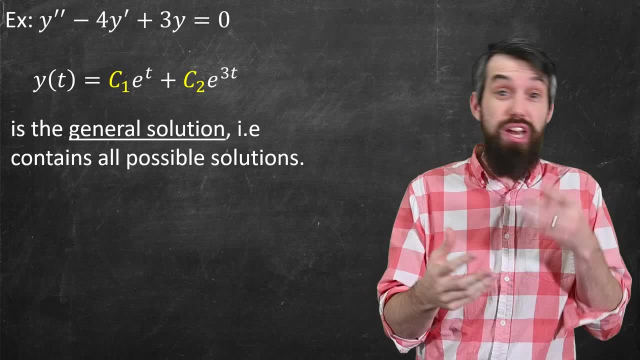 Now to the question of how do you find these solutions like how did I know e to the t and e to the 3t? this is a subject of our course. We are going to study that later on in later videos in this course. 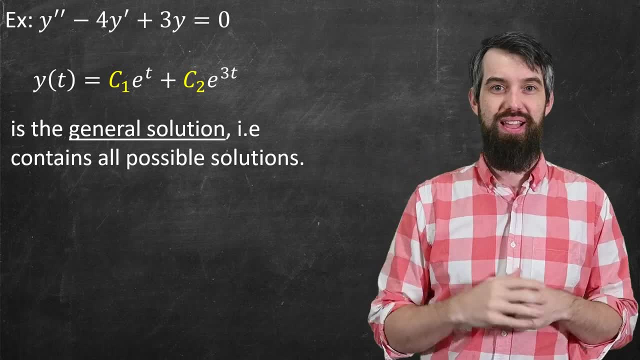 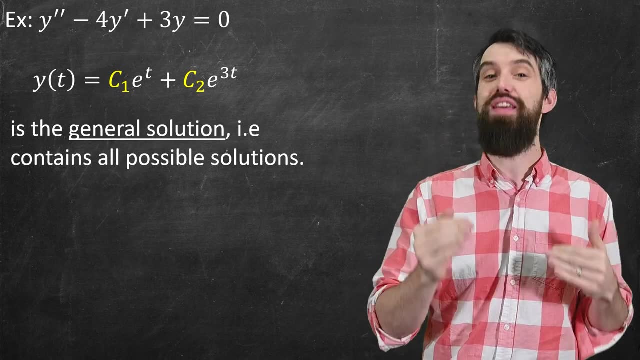 But for now, we can actually use technology to help us out, And the actual technology we're going to use comes from- and I'm very proud to say it- the first official sponsor of this math channel, which is Maple. What I can do with Maple Calculator. 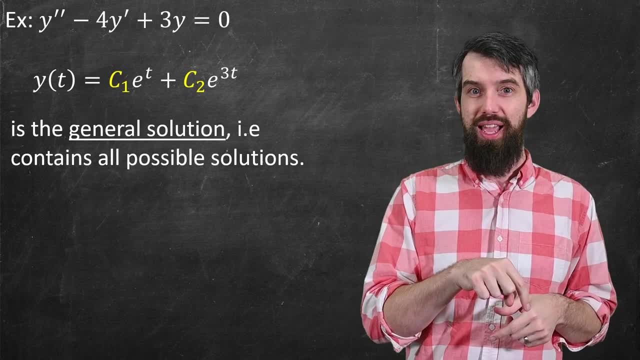 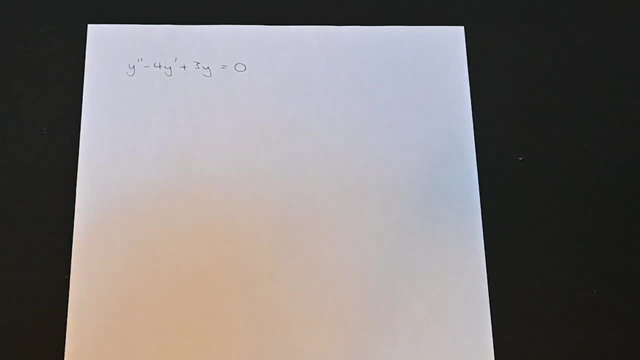 which is an app that you can install on your phone and the links are down in the description, is: I can just handwrite out the differential equation that I'm trying to study. So I can handwrite out: y, double prime minus 4y, prime plus 3y equal to zero. 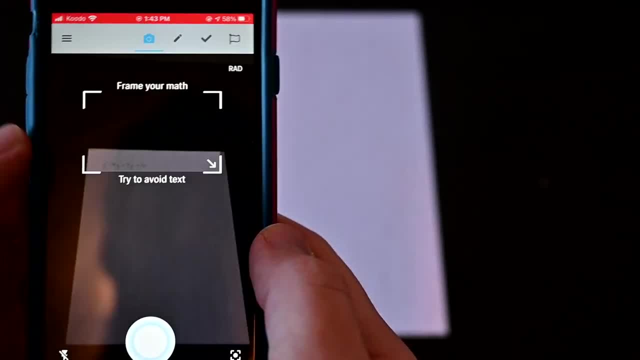 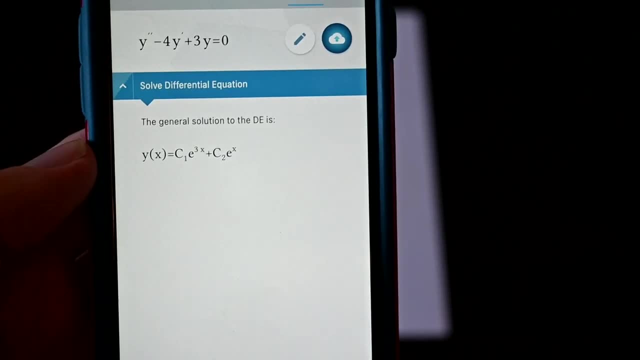 Then if I open the app, I can hit the camera button and I can just take a picture of my equation and the Maple Calculator will interpret it And look what it does. It automatically spits out the general solution to this differential equation. 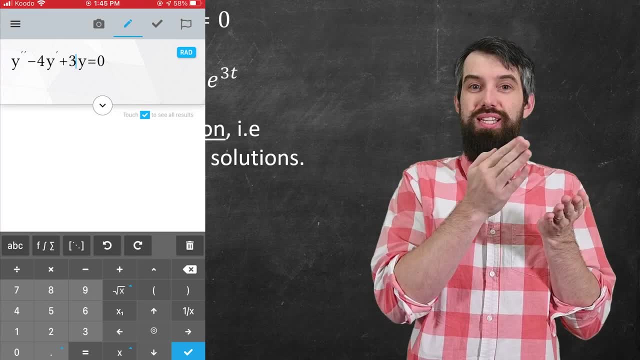 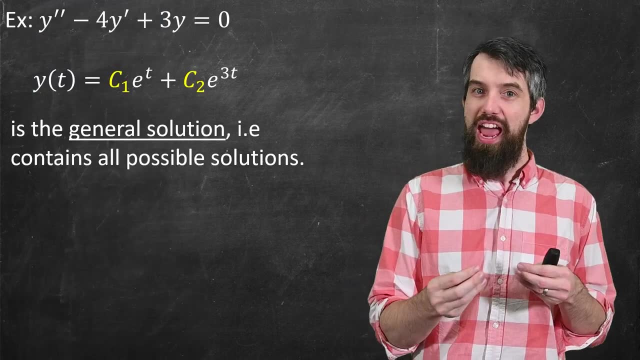 If you didn't want to bother with taking a photo. it's also true. It's totally fine for you to type it in and to change the constants and see what the solutions are to any differential equations that you're interested in. And it's nice to know that, according to the Maple Calculator, 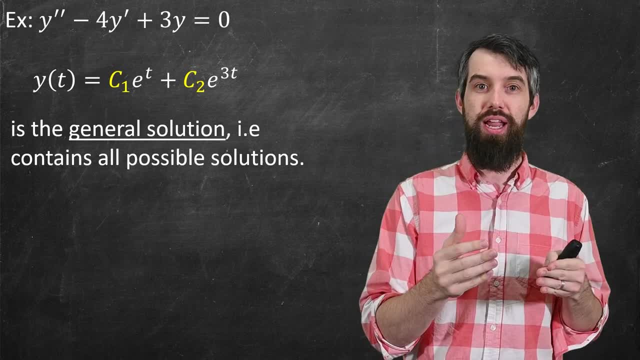 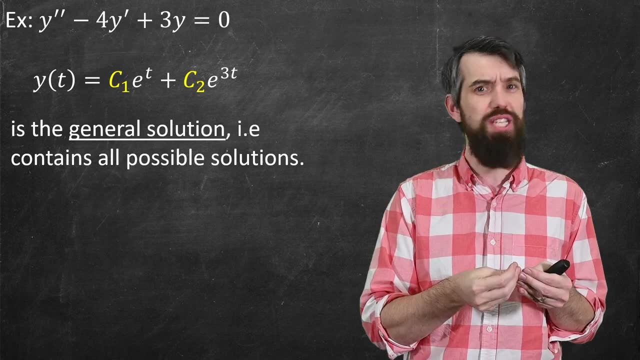 this is all of the solutions. This is the general solution. Indeed, there's going to be a lot of theory that we'll develop later in the course as to how many solutions a different type of equation can have, And it's going to be very intimately connected to the order of the differential equation. 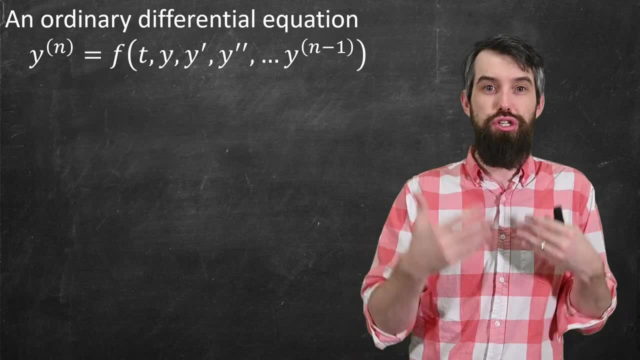 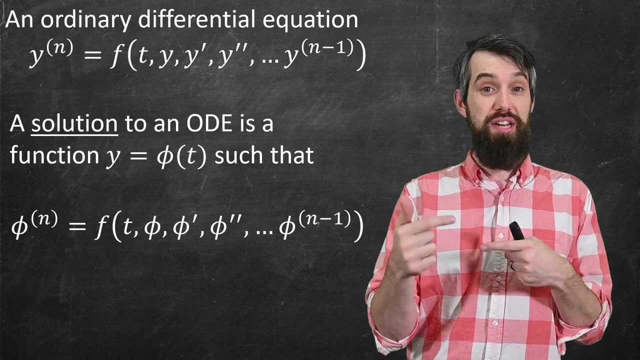 Okay, so let's define this a bit more precisely. Now I want to talk about the solution to an ordinary differential equation. So I'll put up my generic ordinary differential equation And then a solution to an ordinary differential equation. is you telling me a specific function? 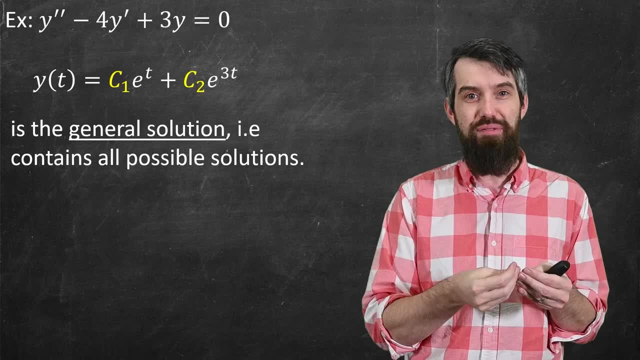 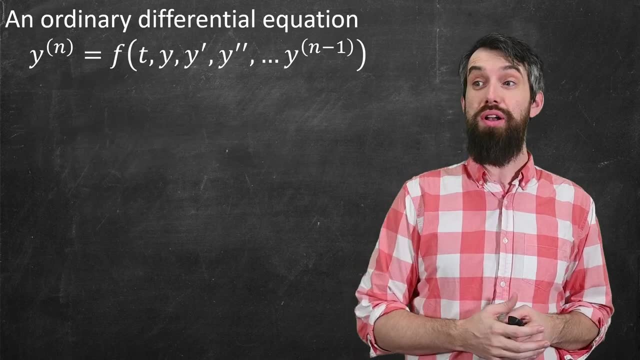 to how many solutions a different type of equation can have, and it's going to be very intimately connected to the order of the differential equation. Okay, so let's define this a bit more precisely. Now I want to talk about the solution to an ordinary differential equation. 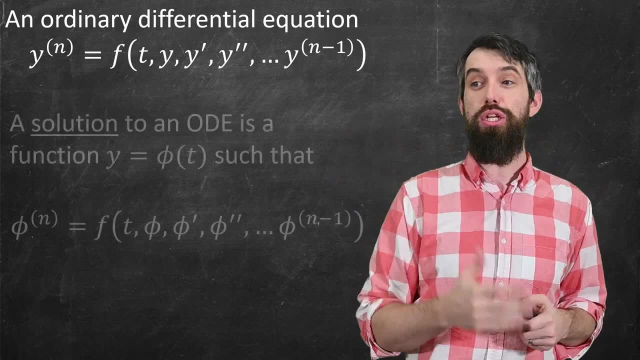 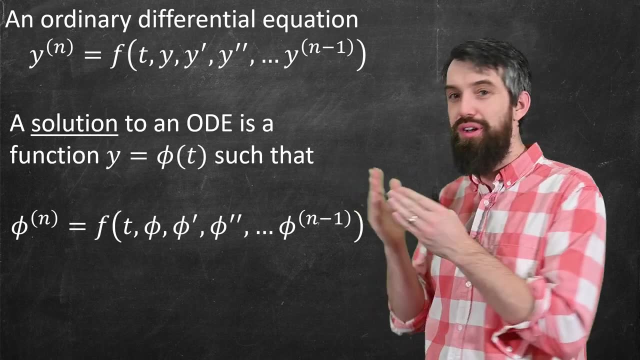 So I'll put up my generic ordinary differential equation and then a solution to an ordinary differential equation. You telling me a specific function. I'm calling it here, for example, phi of t and I'm saying that I'm going to assign y to be that specific function and that specific function when. 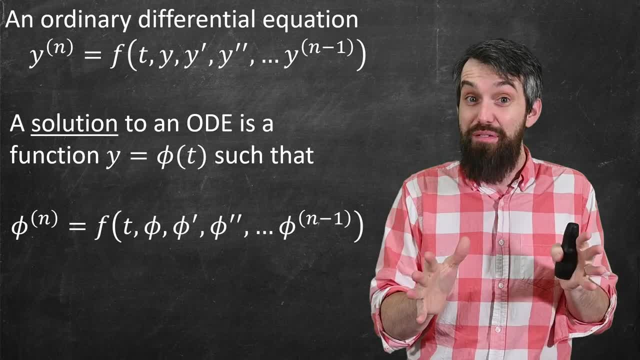 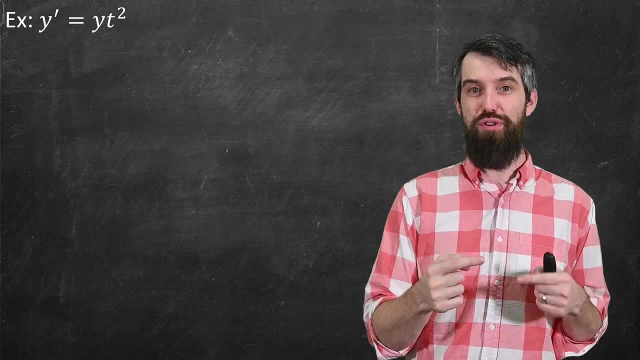 you plug it in everywhere, it's the same equation. just I put phi everywhere instead of y. it solves that equation. So that's our precise definition of a solution. I'm going to give a second example of a differential equation. now, y prime equals y times t squared. 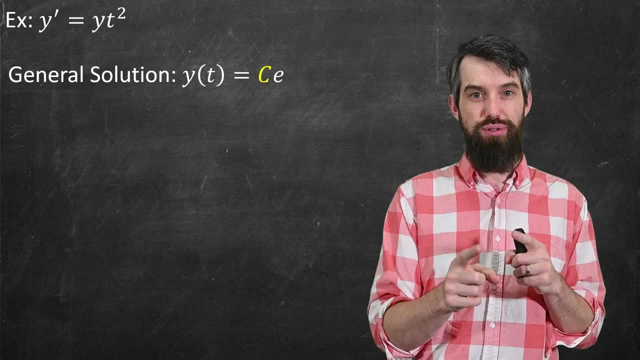 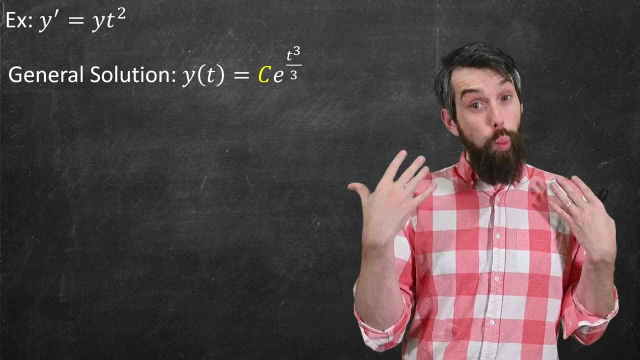 And this is just another differential equation, first order, and it has a general solution: y of t is a constant to t. It's a constant times e to the t cubed divided out by three. So in this case, one infinite family. and again, I'm not going to go into how I solved. 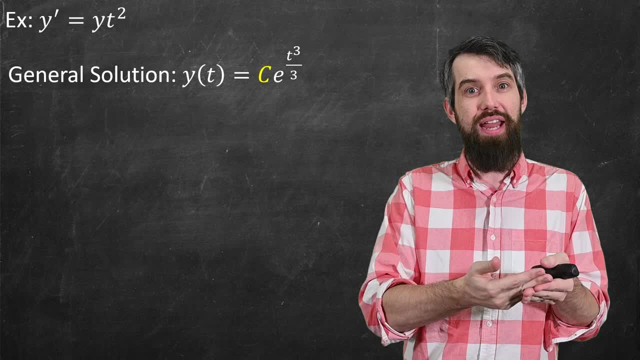 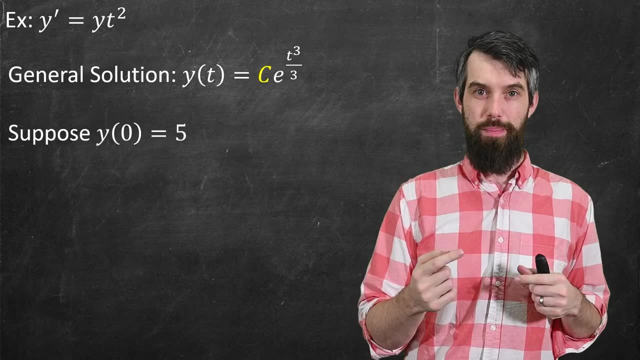 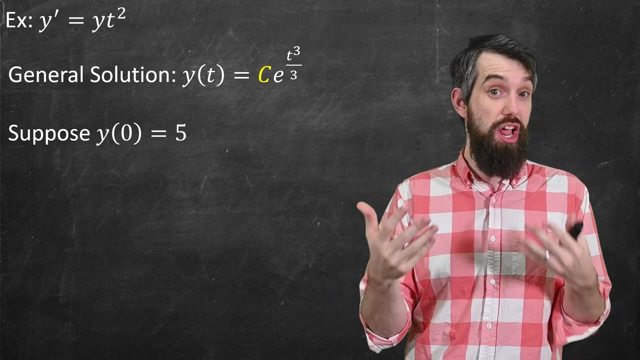 this, but you can verify that it's a solution by taking the derivative, plugging it in and seeing that it works. Now I really want to focus on that c value. So I want to give an extra piece of information. Suppose I told you that at time t equal to zero, y was five, a so-called initial condition. 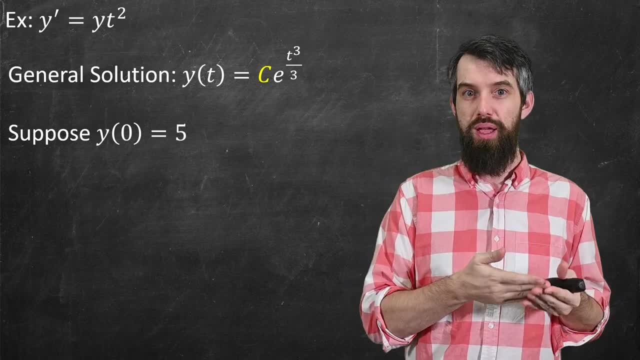 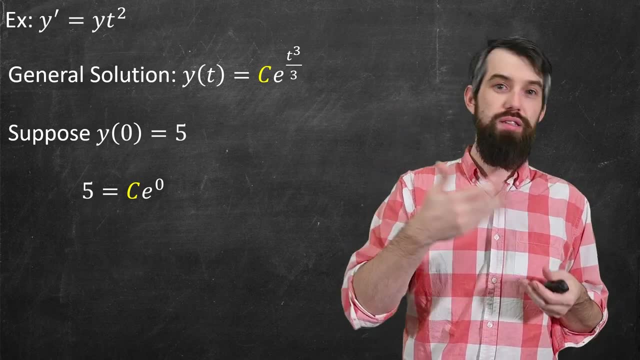 I'm telling you what happens initially at time. t equal to zero. Well, I could plug this in so that would be five on the left-hand side, equal to a constant, e to the zero. if I plug in t equal to zero, e to the zero is one, and so I get that c was. 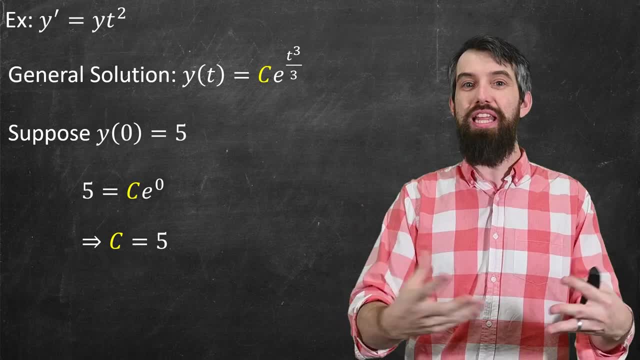 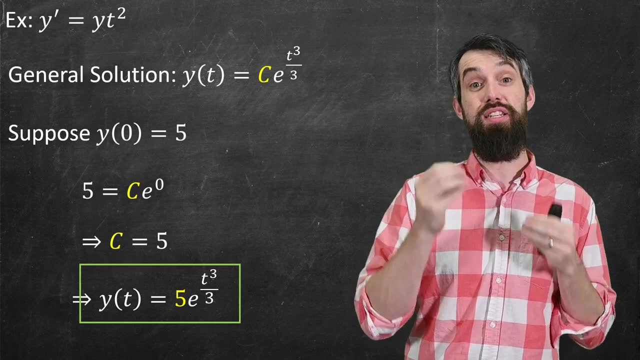 equal to five, And this lets me rewrite what was originally a general condition with an arbitrary constant. I now get a very specific answer. y of t is five. e to the t cubed divided by three. This is referred to as an initial value problem. 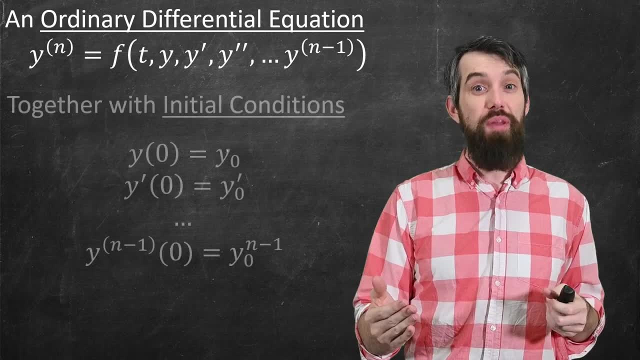 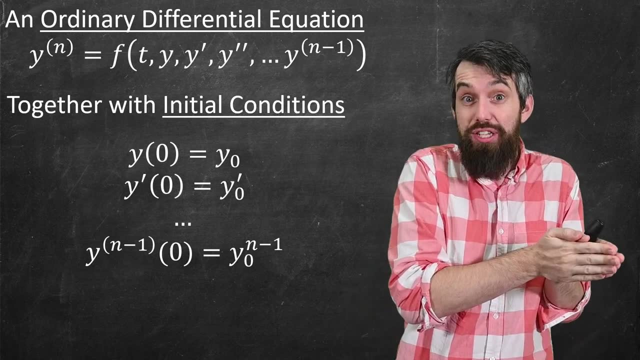 More generally, I would start with my differential equation, as I have, But then, in addition, I would specify initial conditions. What you actually have to do is, if you have an nth-order differential equation, so n derivatives, you have to specify n initial conditions, y, zero, y prime of zero, all the way down. 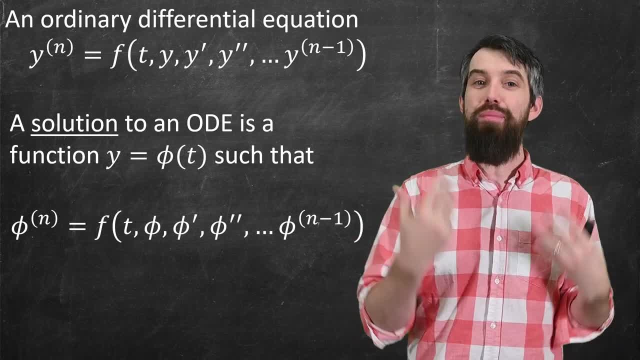 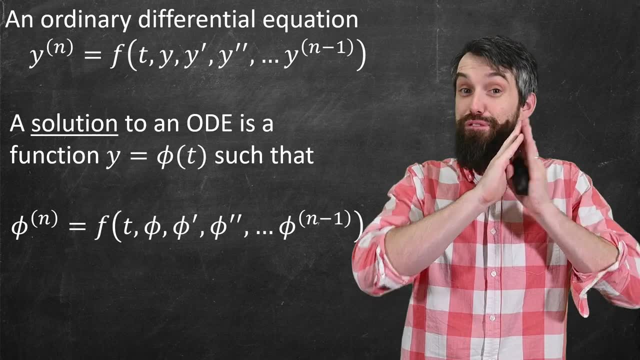 I'm calling it here, for example, phi of t And I'm saying that I'm going to assign y to be that specific function and that specific function. when you plug it in everywhere, it's the same equation, just I put phi everywhere instead of y. 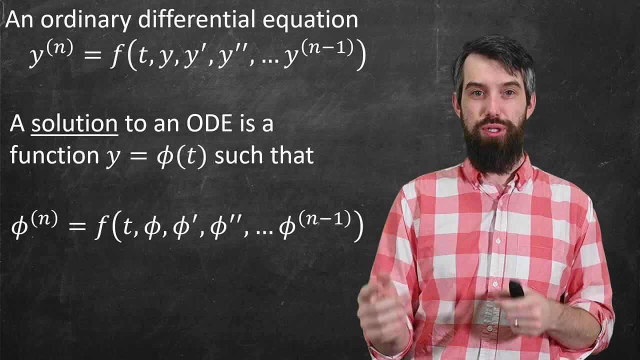 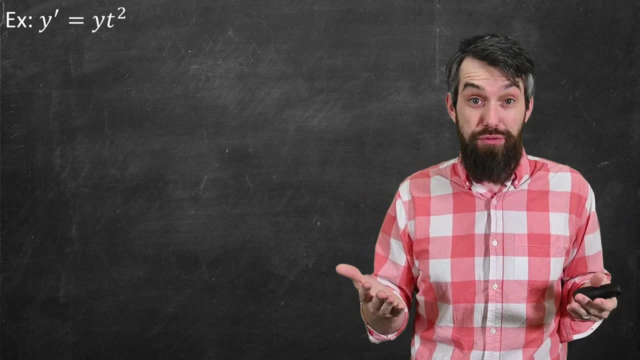 It solves that equation. So that's our precise definition of a solution. I'm going to give a second example of a differential equation: Now y prime equalsлонly. Now y prime equalslonly times t squared. and this is just another differential equation, first order, and it: 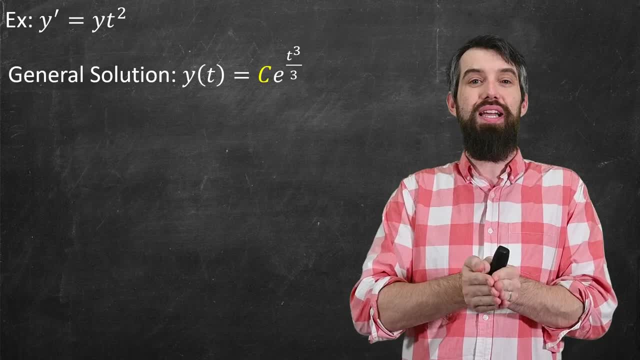 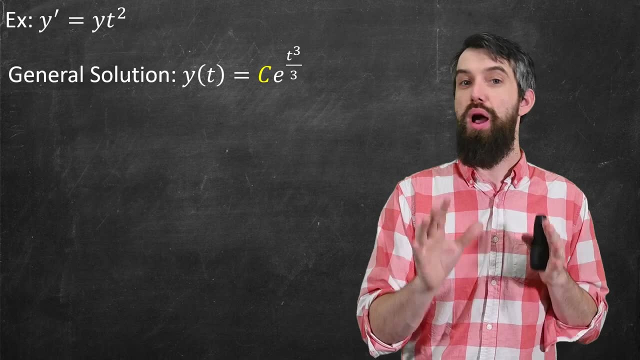 has a general solution. y of t is a constant times e to the t cubed divided out by three, So in this case, one infinite family. and again, I'm not going to go into how I solved this, but you can verify that it's a solution by taking the derivative, plugging it in. 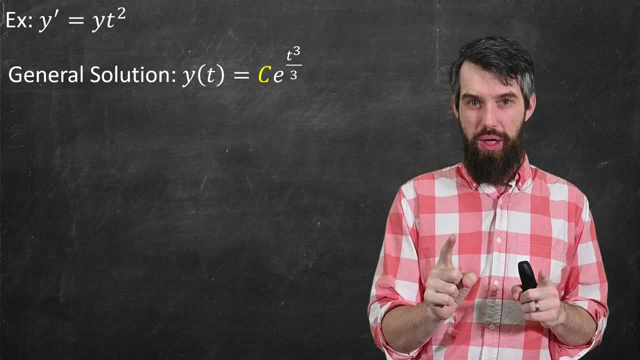 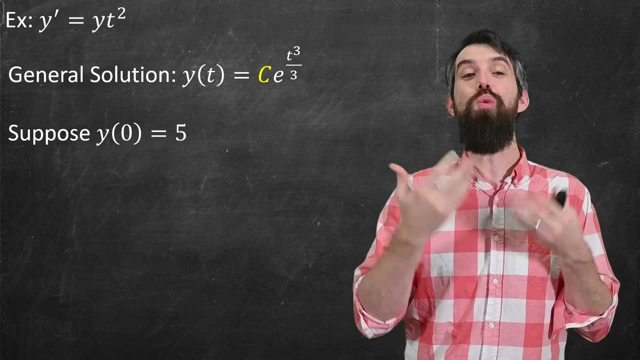 and seeing that it works. Now I really want to focus on that c value. So I want to give an extra piece of information. Suppose I told you that at time t equal to zero, y was five, a so-called initial condition. I'm telling you what happens initially at time t equal to zero. 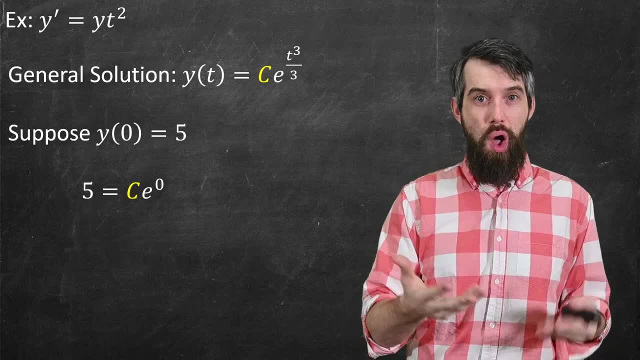 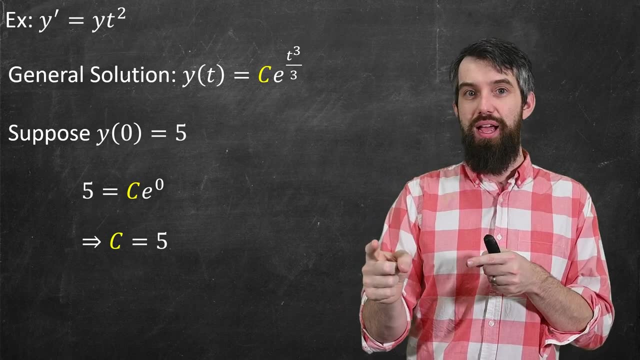 Well, I could plug this in so that would be five on the left-hand side, equal to a constant, e to the zero. if I plug in t equal to zero, e to the zero is one, and so I get that c was equal to five. 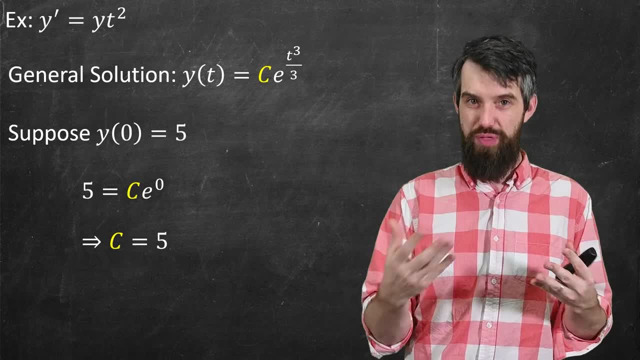 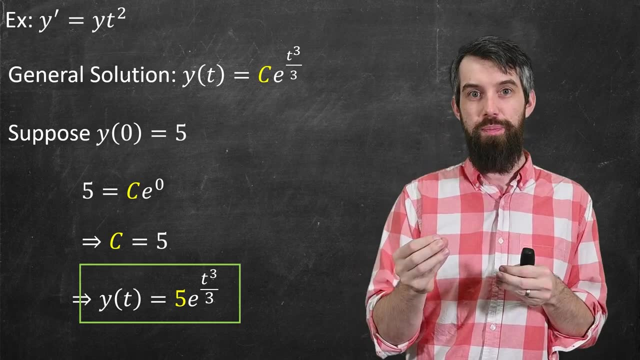 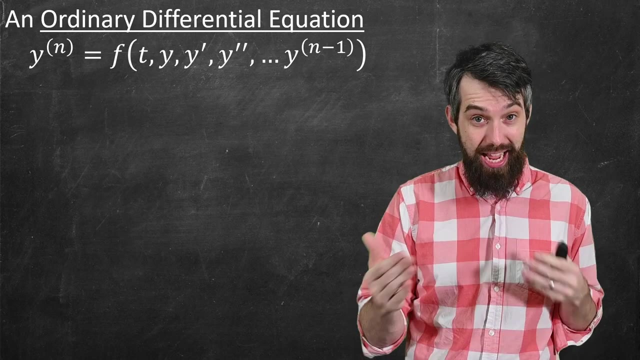 And this lets me rewrite what was originally a general condition with an arbitrary constant. I now get a very specific answer. y of t is five. e to the t cubed divided out by three. This is referred to as an initial value problem. More generally, I would start with my differential equation, as I have, but then in addition, I 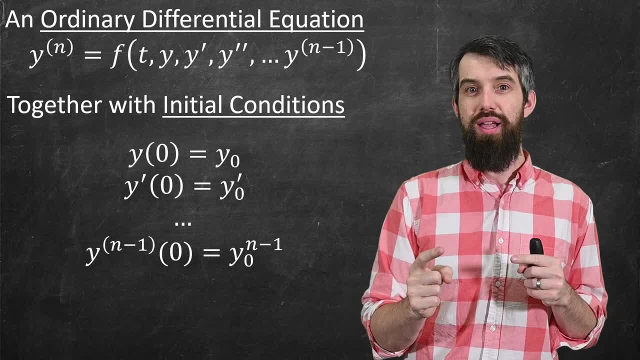 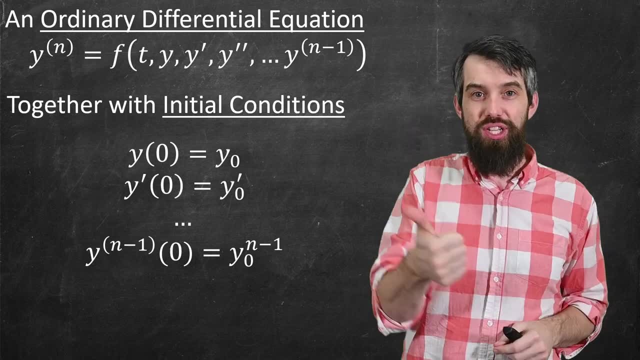 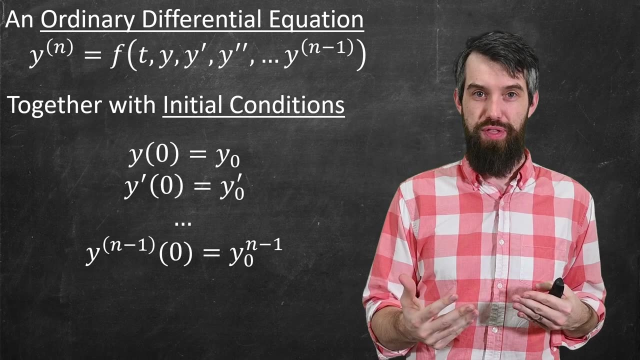 would specify initial conditions. What you actually have to do is, if you have an nth order differential equation, so n derivatives, you have to specify n initial conditions, y, zero, y prime of zero, all the way down to the n minus one-th derivative of y at zero, and you specify the values of those. 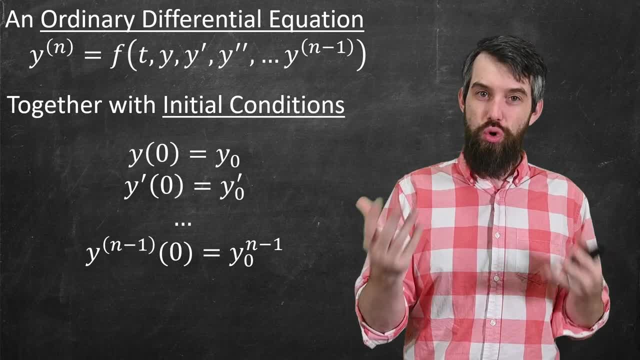 When I say y of zero is one-th order, I'm talking about the derivative of y at zero, and I'm talking about the derivative of y at zero. Why not? Why not is just my shorthand for some constant that will be specified. 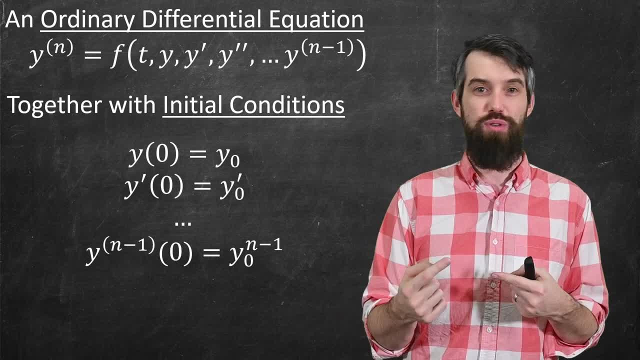 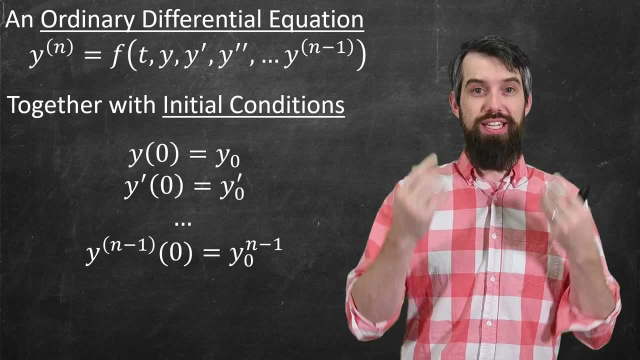 Why not? prime is some constant that will be specified again Whenever I write this little subscript. zero, I call it not, and I just mean by that it is a constant. So I have these initial conditions. I just tell you the values of the function and its